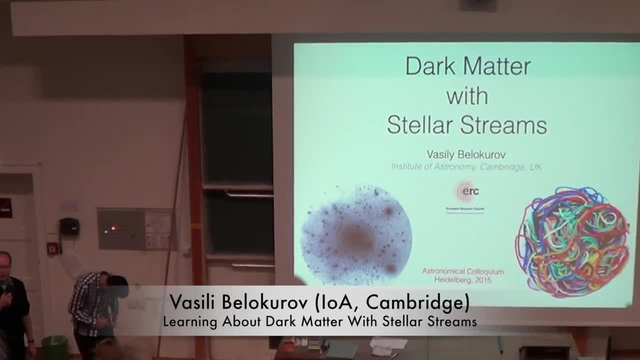 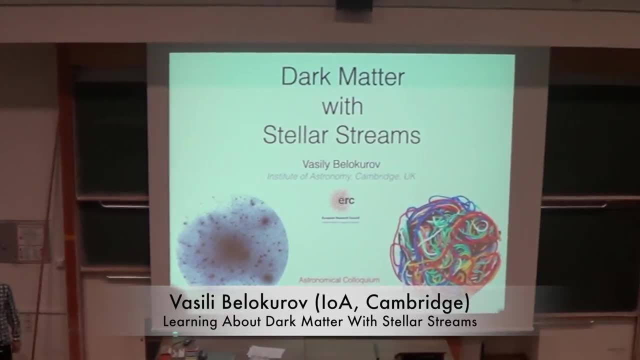 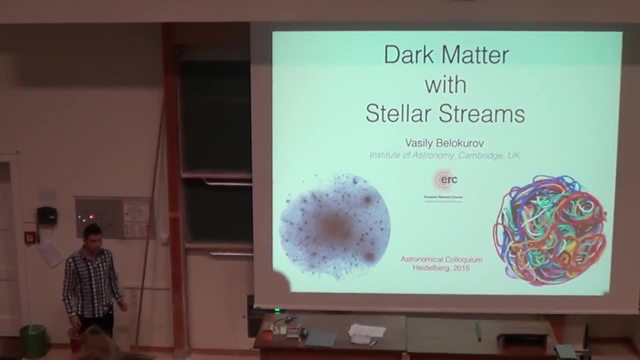 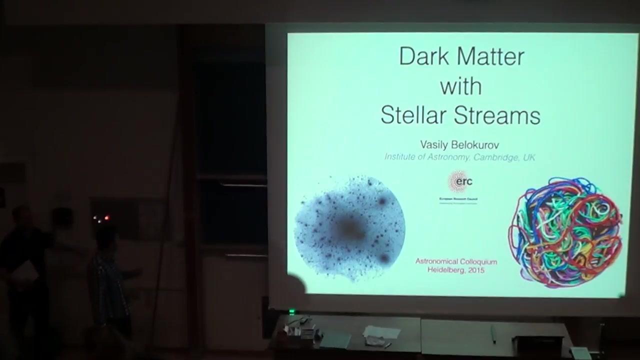 And so today he's going to talk about dark matter with tapestry, So let's welcome him to the high board and the floor is yours. Thank you very much for your words and for the presentation. I'll just go into it straight away, because I know we've run out of time by now. 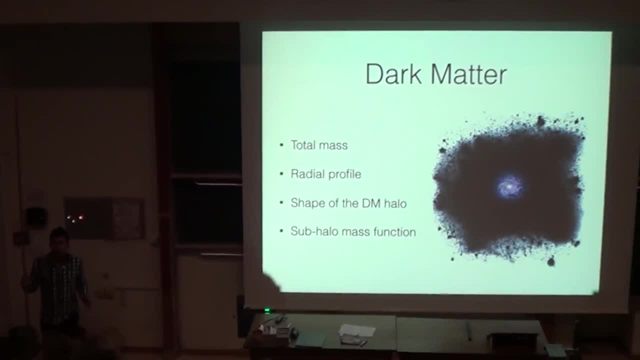 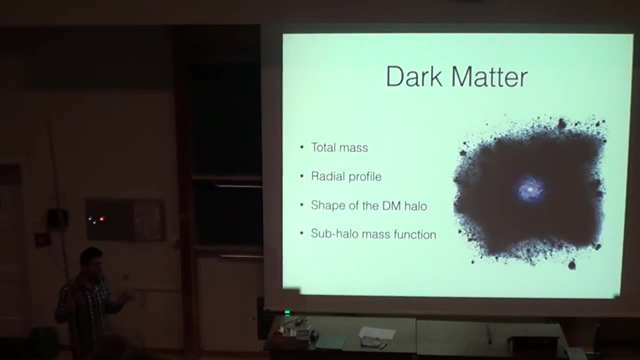 What do we want to know about dark matter? We pretty much want to know most things because it's, at the moment, very mysterious and poorly studied substance. We hope that in the galaxy, in the Milky Way, we can do the best. We hope that the Milky Way is the best equipped laboratory to study dark matter properties. 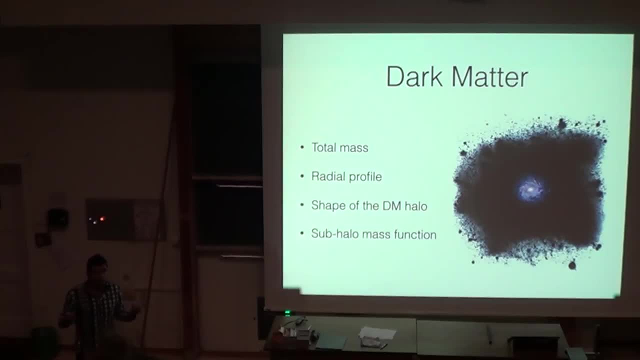 What do we want to learn about Milky Way's dark matter halo? It sounds ridiculous, but at the moment we don't really know the total mass of dark matter in the Milky Way. There isn't any good accuracy. So this is the first thing: to constrain. 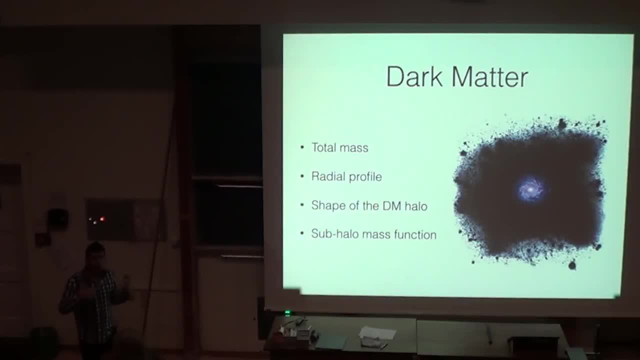 We actually want to do a bit more. We want to also measure the radial profile in the density distribution of dark matter. We also want to figure out what the shape of the dark matter halo is and how it changes with radius- An interesting question that is connected to the nature of dark matter particles itself. 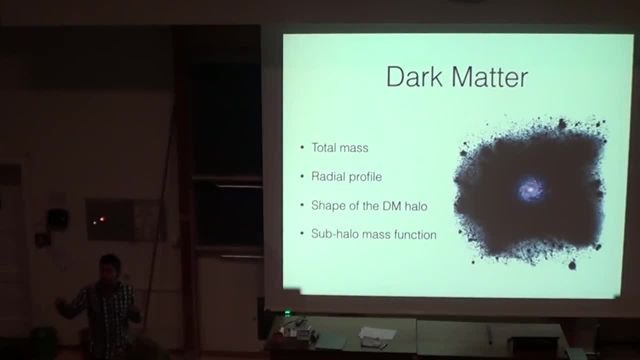 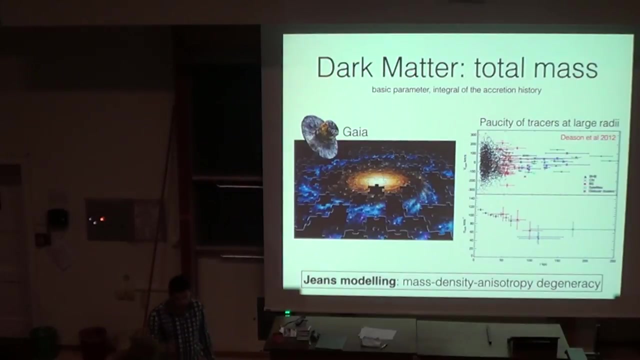 is how far down in mass the sub-halo mass function extends. So we want observational constraints on the dark matter sub-halo mass function. So all these things I propose we can do in the Milky Way with stellar streams, Just to give you a little bit more motivation. why do we care about the mass, for example? 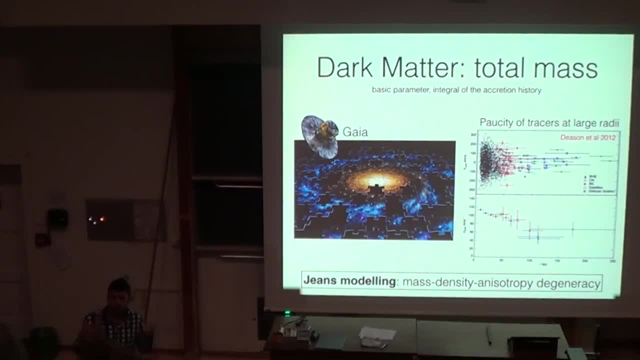 So Gaia is out there measuring positions and brightnesses and motions of billion stars in the galaxy. So we'll have this puzzle of the Milky Way assembled for us eventually with our data, But to be able to compare it to the models that we have of structure formation. 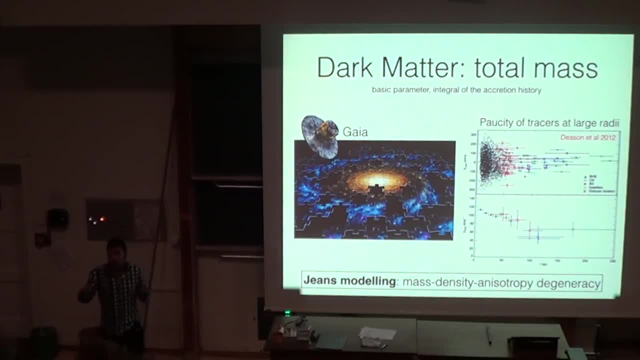 we need to know in what dark matter halo the galaxy leaves. So that's one primary motivation in figuring out the total mass of the galaxy. Of course, the traditional way of measuring the mass in the Milky Way is through spherical genes modeling. You can make it less spherical if you want. 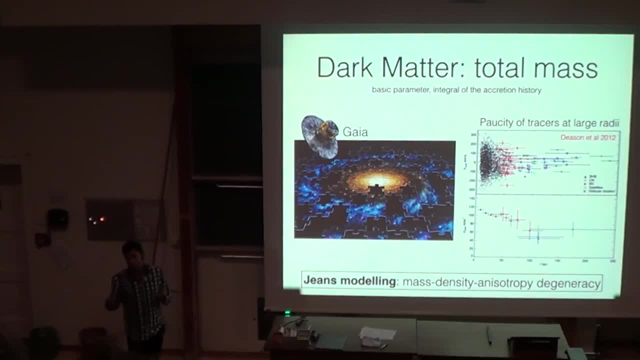 But it's genes modeling nonetheless, And there are problems with it. There is a well-known anisotropy, where you have to know very well the density of your tracers and I'm sorry, I don't speak- degeneracy, Where you have to know the density of your tracers, and anisotropy of their orbits. 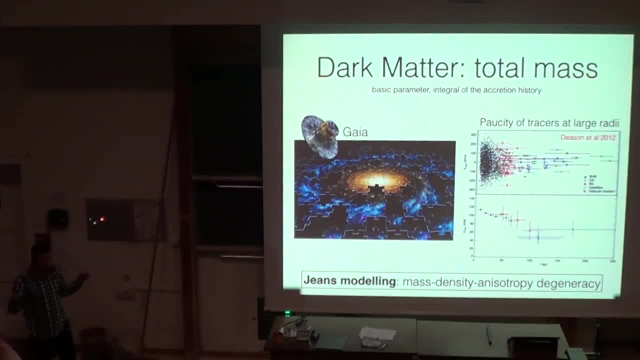 if you want to measure the mass, It turns out, to begin with, there are not so many tracers to measure the mass, So the I'm going to use this interesting pointer. I like this one. So this is the galactocentric distance. 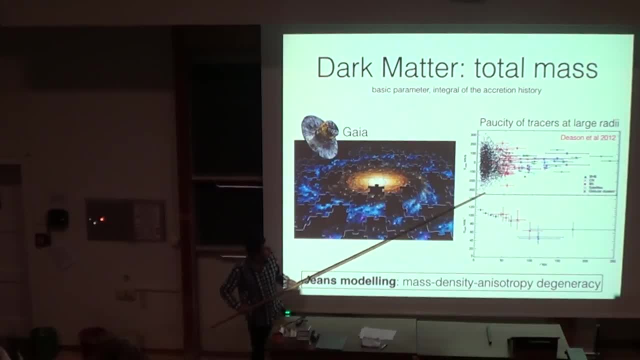 and this is the velocity of the tracer, line-of-sight velocity. You can see that past 40 or so kiloparsecs the density of tracers dropped dramatically. And that's all we have available to constrain the mass. And of course the virial radius is off the plot. 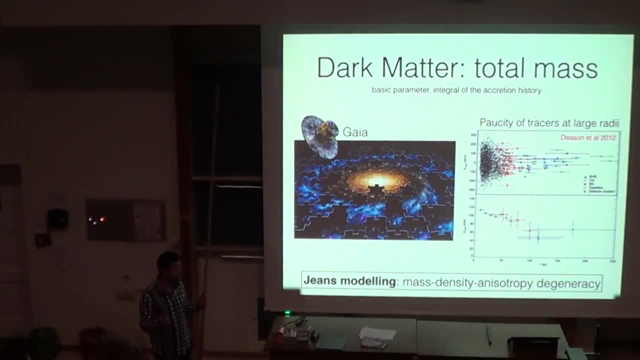 So that's why genes modeling is tough in the galaxy, But, moreover, we don't actually know, because we have so few tracers. we don't actually know what the density distribution is And, of course, we have no idea what the anisotropy of the orbits is. 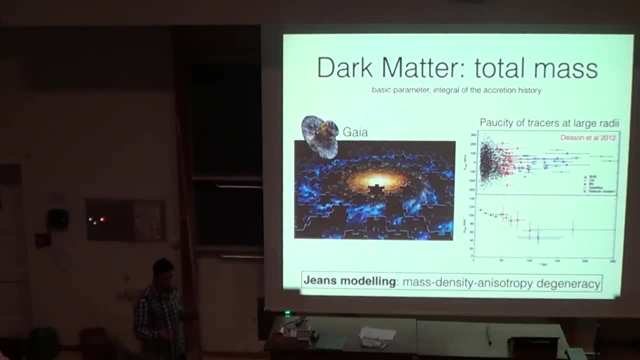 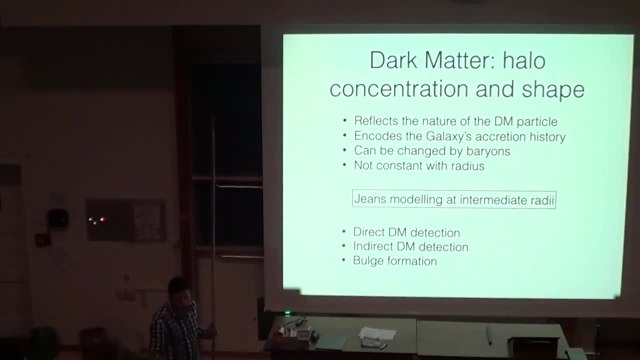 So we have to guess that. So we need a better tool than genes modeling to constrain the total mass of the Milky Way. We want to know the dark matter halos, concentration and shape, And of course the shape also reflects the nature of dark matter particles. 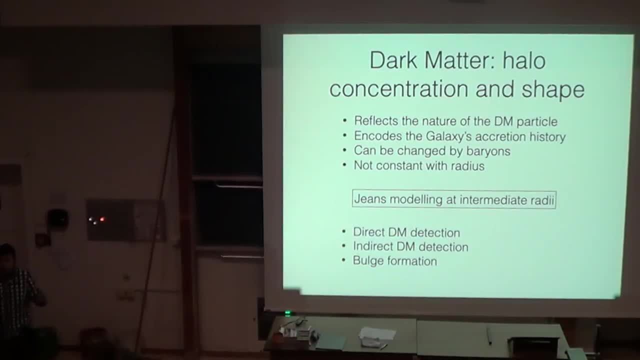 So in Lambeau-Serien we know that most of the halos we have created in the computer look quite prolate. Of course the shape and the radial profile also impose the accretion history which we also came to know what the mass accretion history was on the Milky Way galaxy. 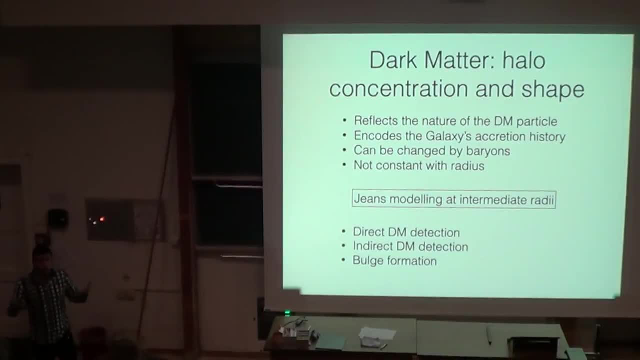 The complication here is that the dark matter distribution, the radial profile and its shape must have been changed, Shaped, reshaped by the invariant feedback, And of course, baryons can drag dark matter with it and make it more concentrated or puffed up. 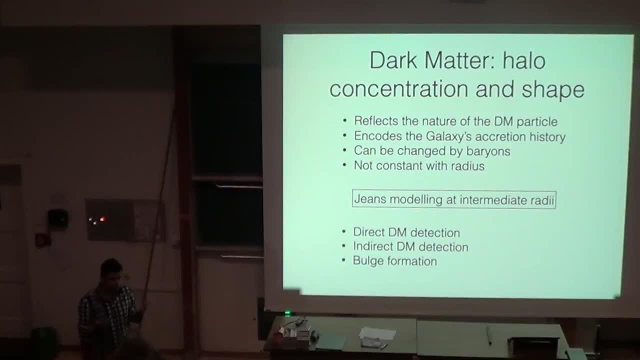 So we want to understand how this coupling happens And of course, to begin with the shape was not constant with radius, But by influence of baryons onto dark matter it's now definitely not constant with radius, So it's changing from the galactic center to the outskirts. 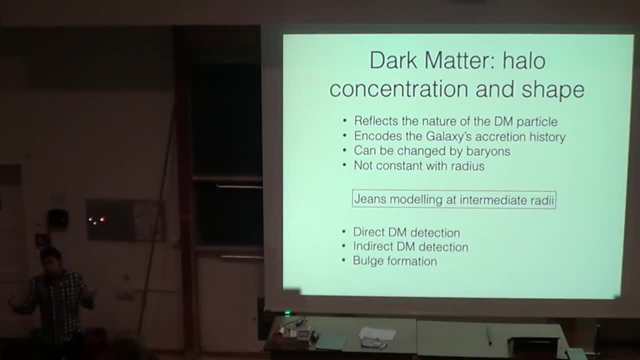 So we want to measure that too, And knowing the dark matter density as a function of radius is important if we want to have any hope to have successful direct detection experiments or indirect epidark matter annihilation probes, If we want to understand why the galaxy formed a bulge. 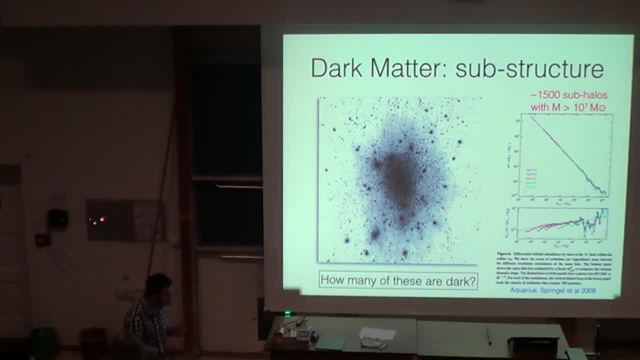 or didn't form any prominent bulge at all. We know that if we take the cosmic microwave background and we use the initial conditions that we have frozen for us in the Earth's universe and run forward our structure formation simulations to action zero, that's what we end up with. 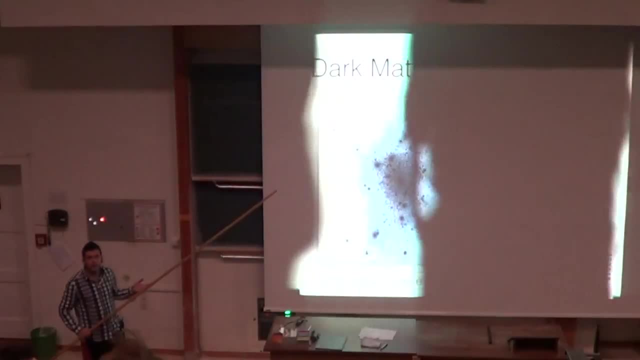 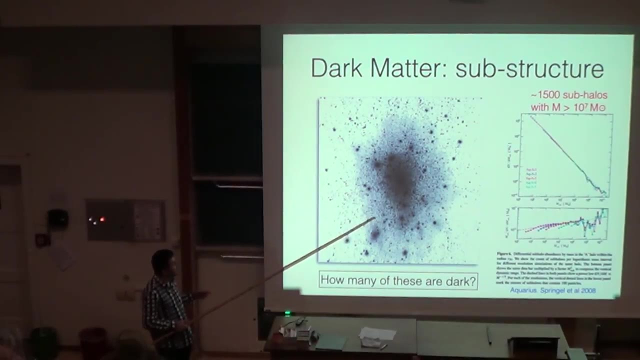 for the Milky Way. It's pretty dark, But it fills a high list of structures. You see that these small subhalos that form the Earth's universe manage to survive to today's epoch and they're still intact, bound orbiting the Milky Way halo. 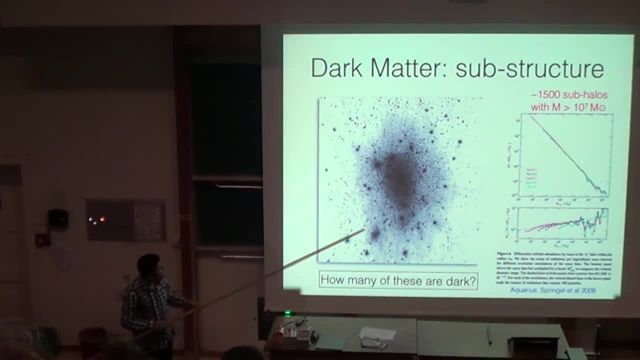 So there is this huge structure, this cloud of dark matter. within it contains swarms of smaller dark matter subhalos, and we have an idea of what the mass function which is shown on the right panel of these subhalos should be, But we actually want an observation. 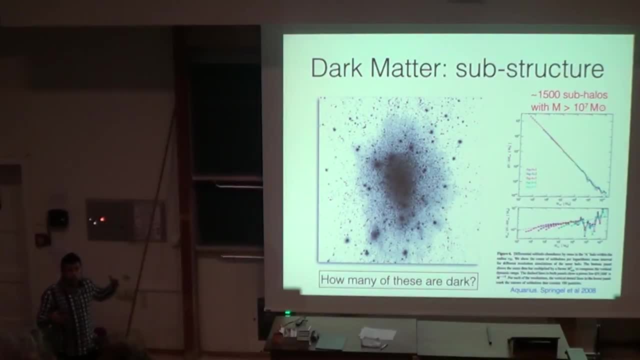 of that. Some of these subhalos will have accreted and cooled enough gas to form stars from it, and so they will host a dwarf galaxy inside them, But probably not all. For example, we think that potential hosts host sites for dwarf galaxies. 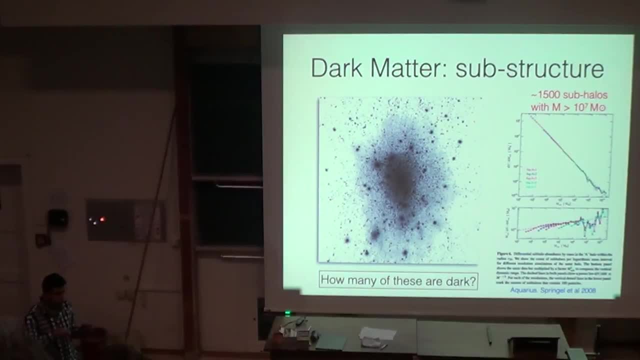 in the Milky Way. these are the subhalos that today have virial masses in excess of 10 to the 7 solar masses. So of these we have a quarter of a thousand and a thousand and a half, We think by looking at the dwarf galaxy sensors. around us that we have at least a hundred dwarf galaxies, maybe slightly more, Which means that more than a half, or potentially much more than a half, of these thousand and a half subhalos with masses in excess of 10 to the 7 will be completely gone. 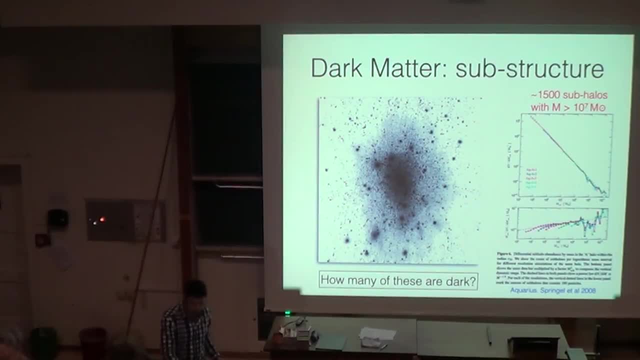 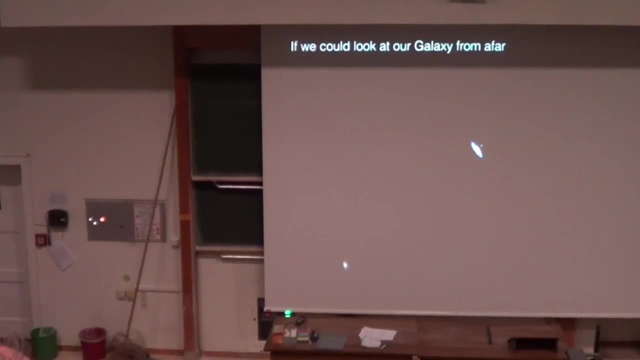 If that's true, we want to find them. So if we could look at our own galaxy from afar, that's how it would look like. and this is, of course, our nearest neighbor, Andromeda. What we've learned recently is that it is surrounded by this mess of the stellar halo. 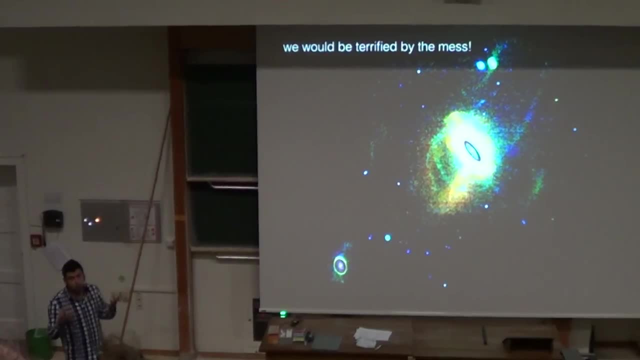 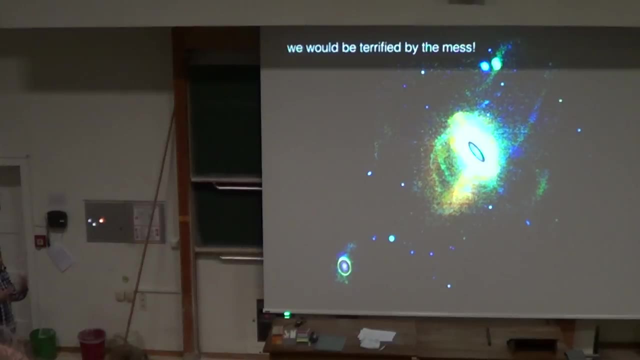 and it's messy, because what it is made of is the debris- stellar debris- from dwarf galaxies that fell into the potential potential of Andromeda, disrupted, and then their stars are now part of the stellar halo that is highly substructured. These are density of stars. 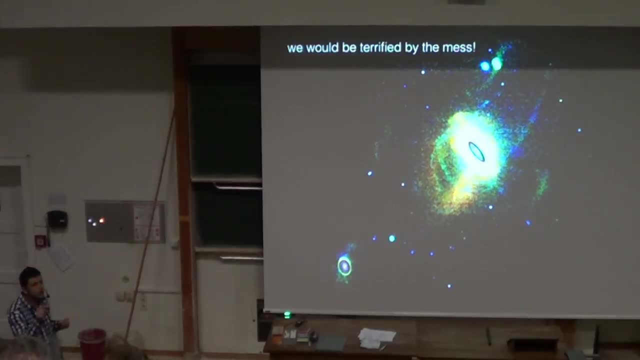 and they're telecoded by their metallicity. So each star had to be detected, its colors had to be measured and the colors were turned into metallicity estimate, and then this map was built. So we believe that something like this exists around the Milky Way. 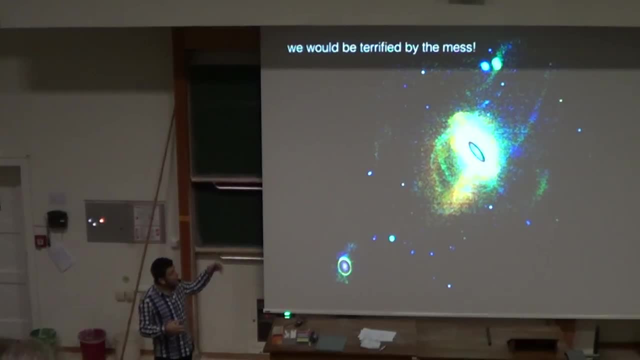 We want to use this stream to measure these streams and these shells, these substructures, to measure the properties of the dark matter. So the stars in the streams. they are tracers of the gravitational potential, and the gravitational potential of the mass budget is then made by the dark matter. 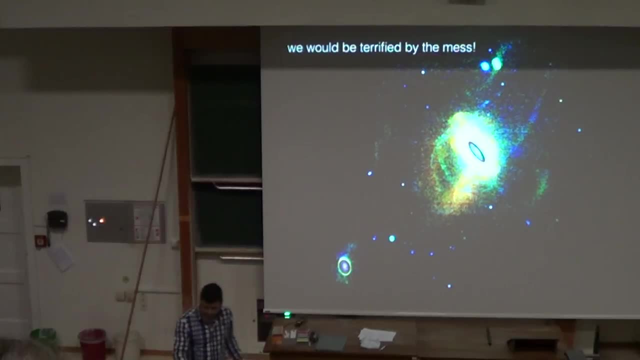 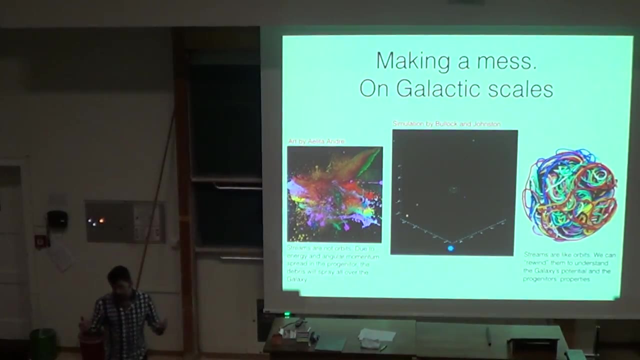 to which the stars contribute almost nothing. We have a very good idea how to make a stellar halo by disrupting dwarf galaxies. Here is a very old simulation of stellar halo formation by Willock and Johnston, in which they had a constant potential into which they threw. 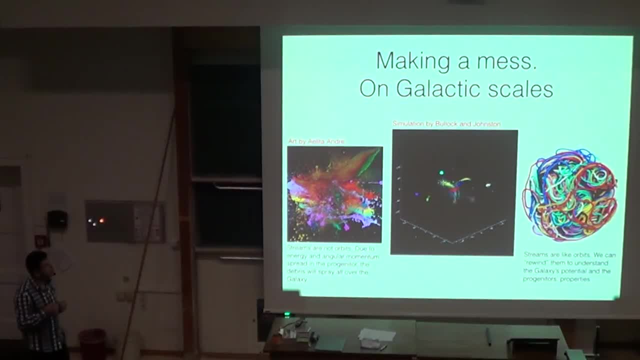 particle represented live halos. they disrupted those and the stars from those dwarf galaxies. calculated by the origin by the progenitor formed the debris, the stellar halo around the Milky Way, which is not shown in this animation. When you see the streams, there are two things that are important. 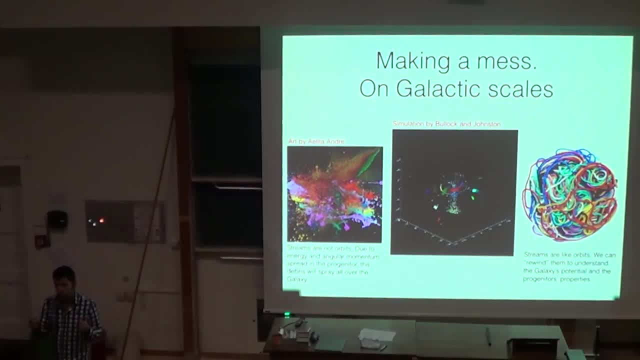 First streams reveal orbits to us. So in principle, if we can find a stream, we can rewind it back, and in rewinding it back we can learn about the underlying gravitational potential. So there is a direct link to the orbit of the progenitor, essentially, 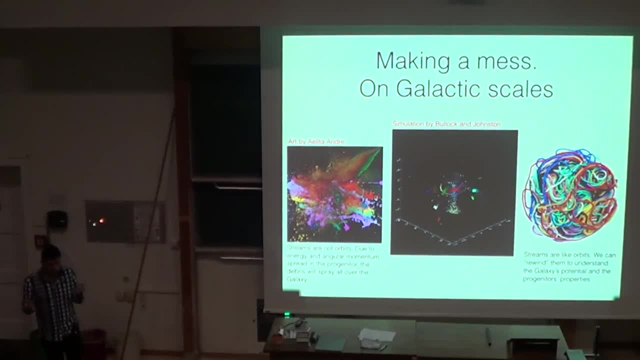 and the orbit of the progenitor is drawn for us on the sky. However, streams are not orbits. There is a spread of energies- negative momentum- to the stars that live on the progenitor, And this means when the stars leave the progenitor, the orbits will be slightly different. 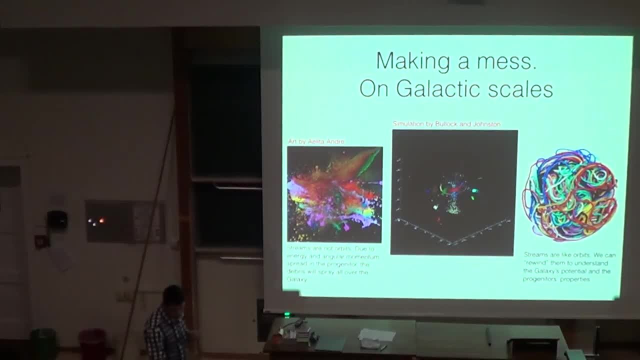 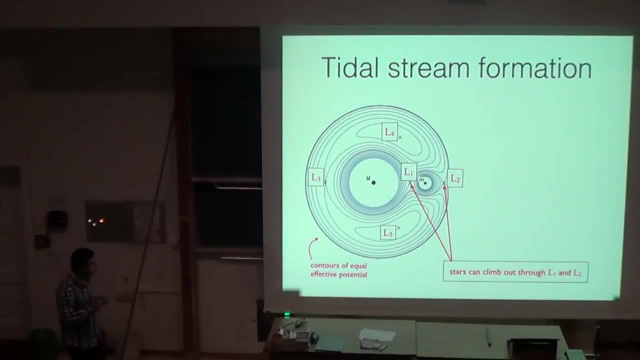 from the progenitor and from each other. So let me just remind you how stellar streams form. So here is the familiar picture of contours of effective potentials in a two-body system, say Sun and the Earth, and there are Lagrange points of special meters, the Lagrange points 1 and 2. around the satellite. So stars- if I replace now the Sun and the Earth with the galaxy and its satellite stars in the satellite can climb out of the satellite through Lagrange 1 and Lagrange 2.. So the question: why would stars decide to climb out? 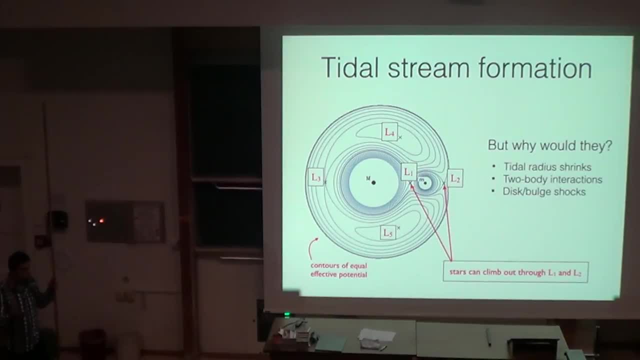 and there are many different reasons that can compel them to go through Lagrange 1 and Lagrange 2.. So as the galaxy, the dwarf galaxy, the satellite orbits the host, as it finds itself closer to the galactic center or to the disk, its stellar radius will shrink. 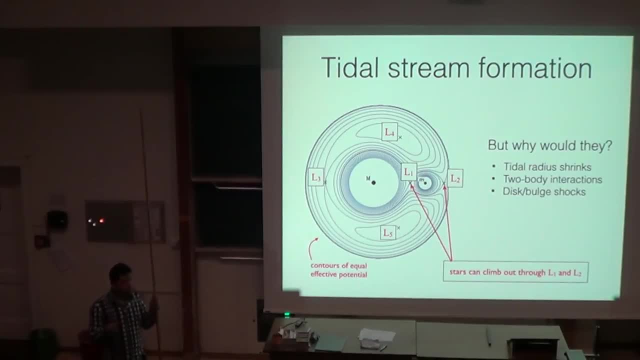 so the stars will find themselves closer to Lagrange 1 and Lagrange 2. if it was a globular cluster, the satellite was a globular cluster. the stars can be thrown out to the periphery to the Lagrange points by two-body interactions and, of course, 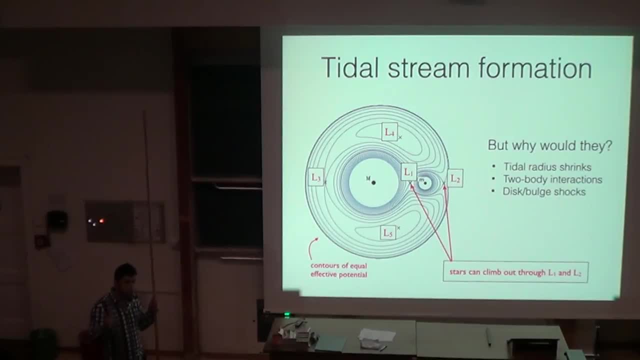 as the satellite goes through the disk and here it bulges. it is shock-heated, so the stars again are pumped to the periphery. So the stars that find themselves near L1 and L2 can leave the satellite and some of them will choose to leave. 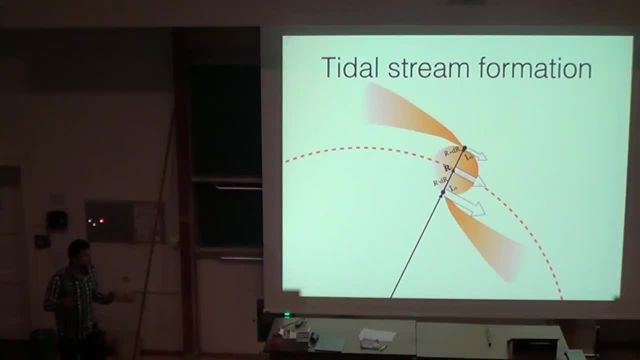 and those that have left will form stellar streams. One stellar stream will be formed from stars that left the progenitor. so this is the satellite galaxy that orbits the host, who is centered somewhere under the floor. so the stars that left for Lagrange 2 will have high energies. 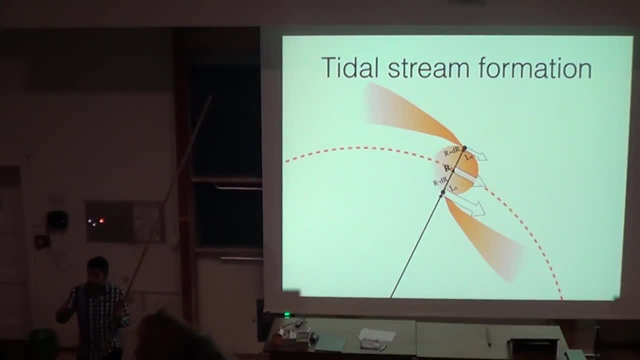 and high angular momentum. compared to the progenitor, they will be on high orbits. so the orbital periods on high orbits are long enough. so they will start to trail behind the progenitor. so similar pictures banded through: stars that climb off Lagrange 1. they are on lower orbits. 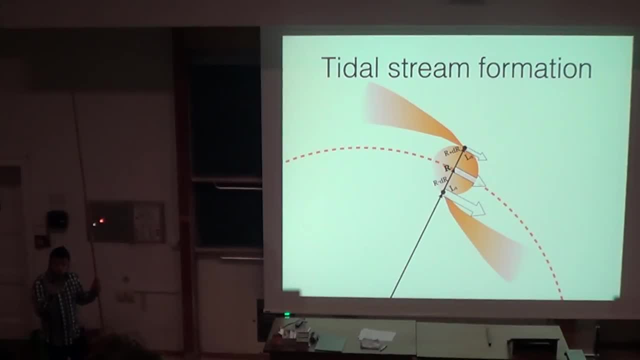 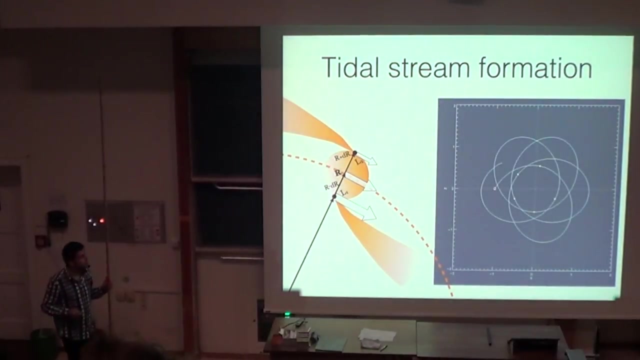 with lower energy and lower angular momentum. those periods are faster, so they will start to leave the progenitor. so two tails will form, one in front and one behind the satellite. so here I am going to illustrate this process by releasing swarms of particles at Lagrange 2 and Lagrange 1. 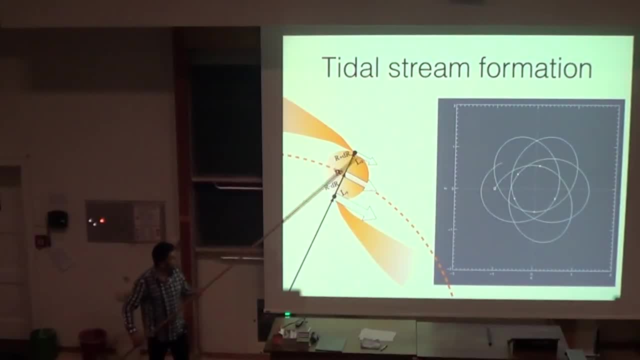 every time the satellite goes through a pericenter. so here is the orbit of the satellite in some molecular potential, and I have marked positions of closest approach to the pericenter and I am going to release Gaussian clouds of particles that have otherwise the same systemic velocity as the progenitor. 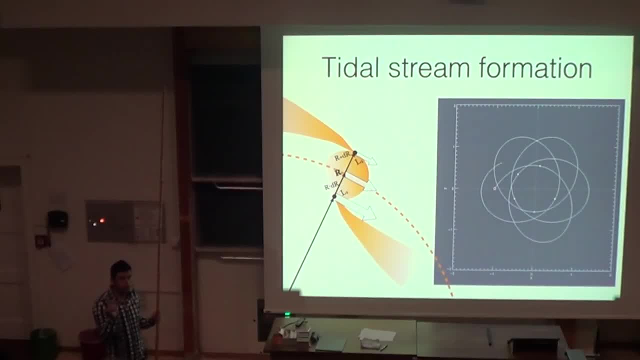 they have small Gaussian velocity dispersion in x and y. and let's see what happens. and I colour code: red is leading and blue is trailing. in the different shapes of red and blue, a different sweeping epoch. you can see that with time the stars redistribute themselves along the orbit of the progenitor. 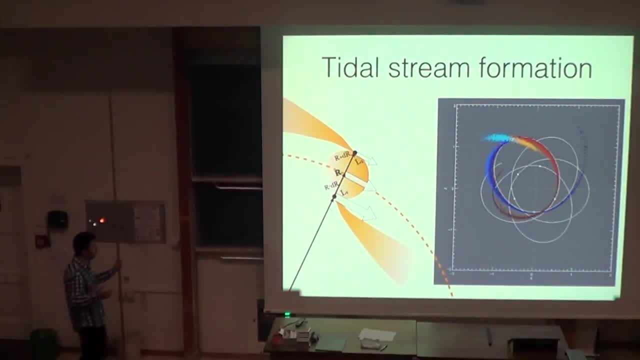 and the orbit of the progenitor is revealed. you can see that the ordering or the type of the release is still encoded in the stream. you can see the colour, shape, planation along the stream so you can see the individual sweeping epochs still discernible. 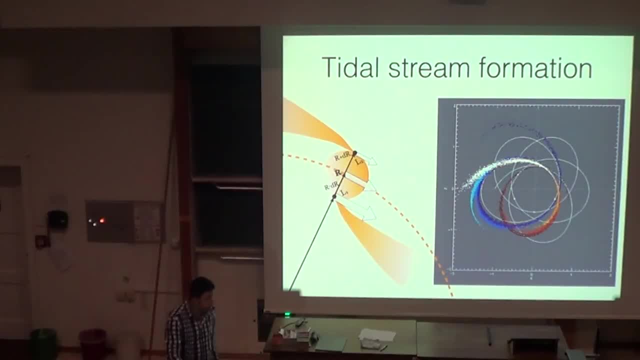 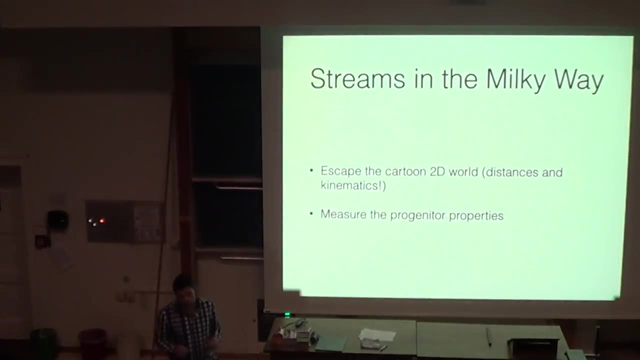 in the stream structure. so that's interesting and you see the individual streamlets start to separate close to the upper centers. for the trailing table, what I showed you earlier was the stellar halo in the Andromeda galaxy. it's beautiful and it's a comprehensive census of streams. 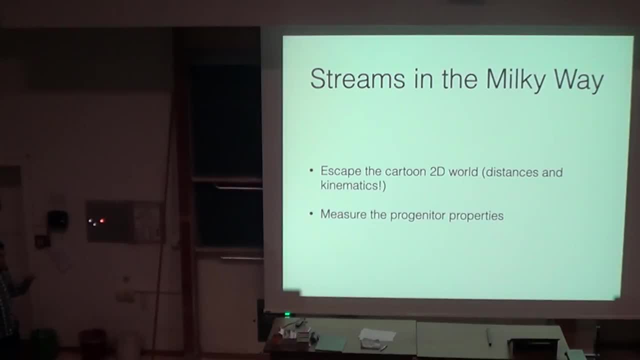 which we can never hope to build in Milky Way, because we see inside the Milky Way. we always have this in the wave, confusing the picture. however, in Andromeda you can never measure very accurate distances along the line of sight. it's also very difficult to follow the streams up. 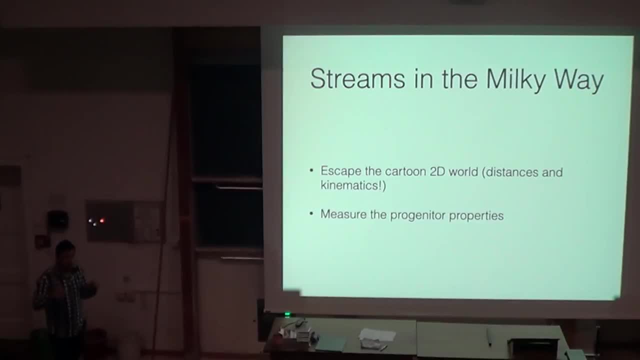 with velocities. however, in the Milky Way, even though we don't see the entirety of the stellar halo, we can measure distances quite accurately. more importantly, we can obtain quite cheaply kinematics. we can obtain line of sight velocities by measuring the structure of stars. now Gaia will measure proper motions. 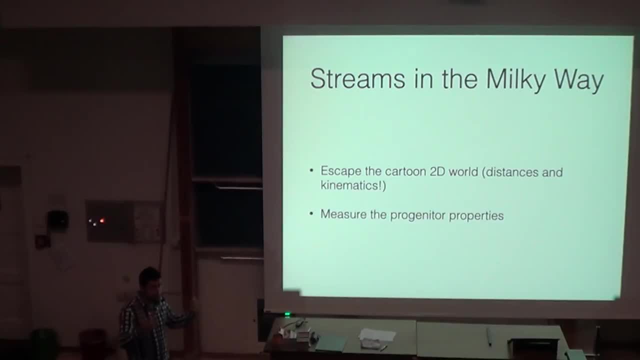 and the OSST will push the proper motion study even further. moreover, we can measure the chemical abundances of the stars so we can understand what the progenitors were. so progenitors represent this class of dwarf galaxies that were formed early on and destroyed, and we don't really 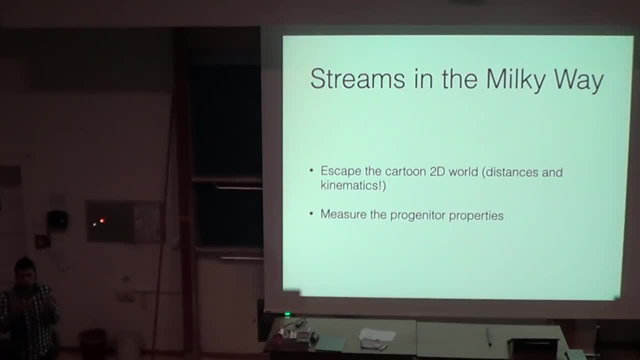 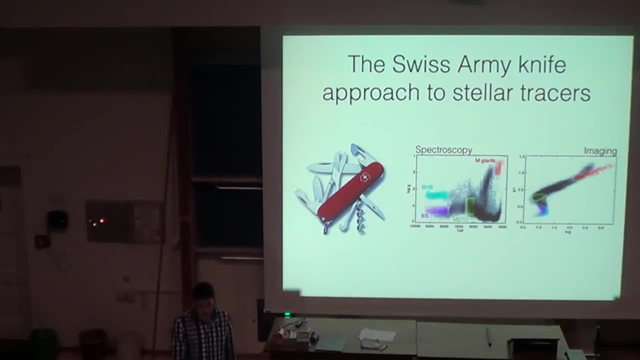 get to study them anymore because they are not intact, but we can learn about the properties for the studies of the stream, which is an interesting subject in its own right. so when we want to study stellar streams, we need to use this kind of Swiss army knife approach. 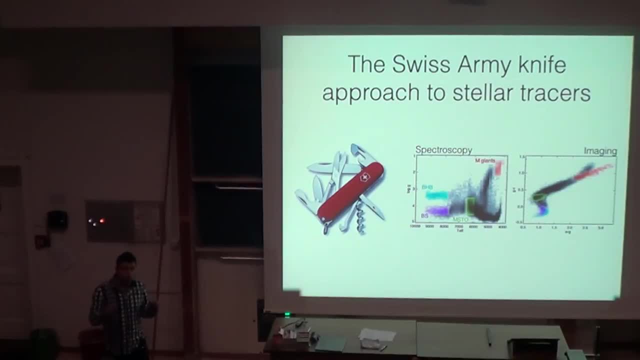 we need to use different tracers, stellar tracers, because different stellar tracers are good for different things. for example, we want to use main sequence turn of stars because they are abundant, because they must defunction of stars peaks and increase its white. they are fast when we hit. 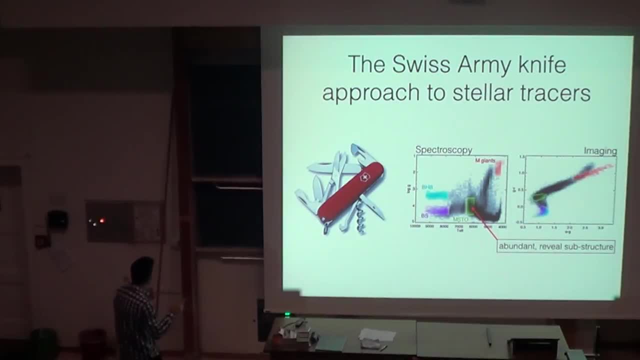 the main sequence, by the way, this particular plot is a density of stars with spectra in the plane of effective temperature and surface gravity. so this is basically a Hersch-von-Russell diagram and these are stars with spectra in the form of planetary database and I've calculated 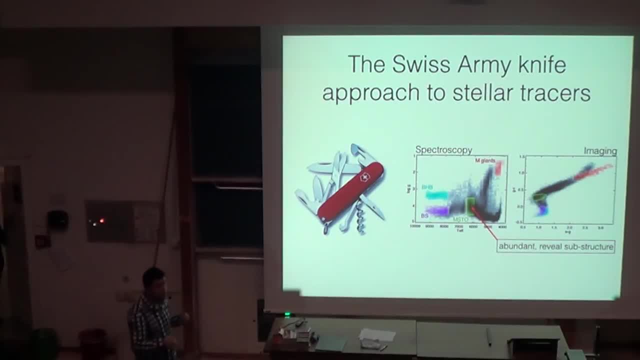 different, interesting, useful stellar tracers that we can take advantage of when we study the stellar halo. so, as I said, most abundant are main sequence and main sequence turn of stars. we can use blue horizontal branch stars because they are good standard candles similar to our libra. 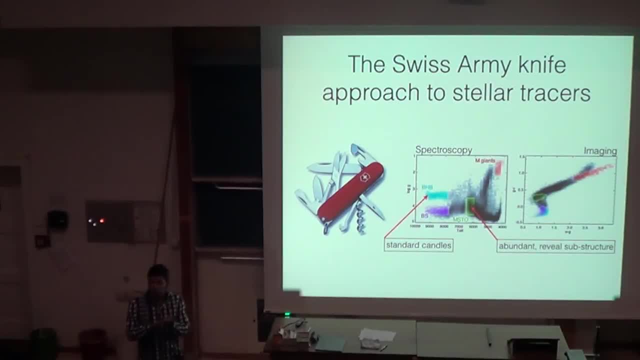 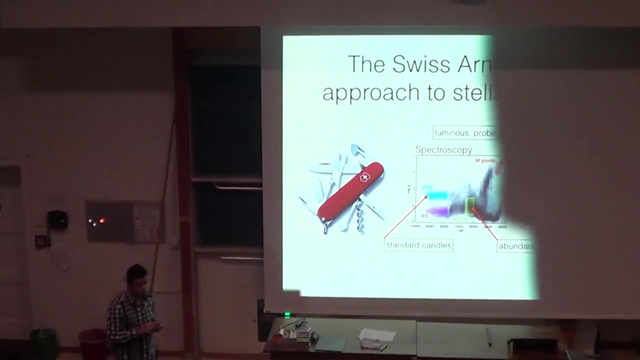 and they are very clean tracers. they are not contaminated by dwarfs or giants. and of course, we can use K-giants and M-giants because they are extremely luminous and they can be luminous so they allow us to reach into the outskirts of the. 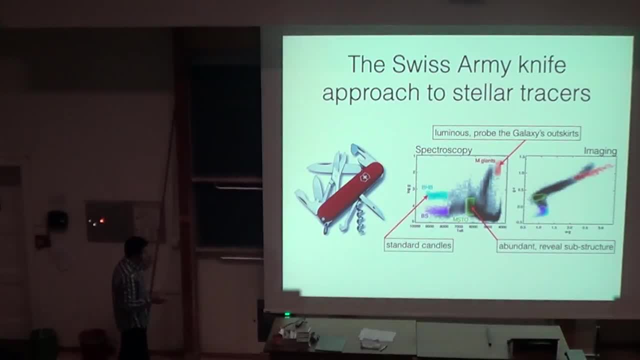 galactic halo. curiously, we can find the same sort of tracers. so this is how easy it is to pick them up with spectroscopy. of course, spectroscopy only exists for a fraction of a percent in the SDSS database. most of the stars have no spectroscopic. 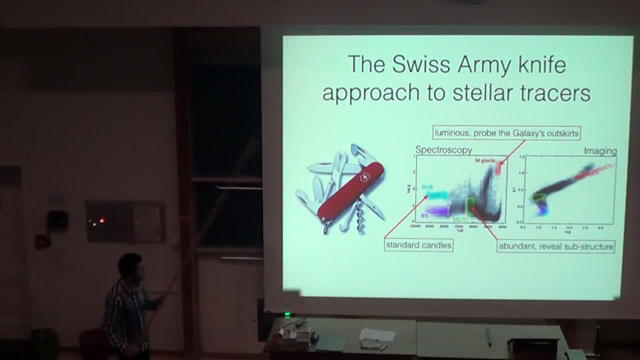 fallout. but it turns out that for this classes of stellar tracers you can also identify them pretty easily with photometry only. so this is now a color plane in which I color coded regions of it according to what stellar tracers live in. so you can see. 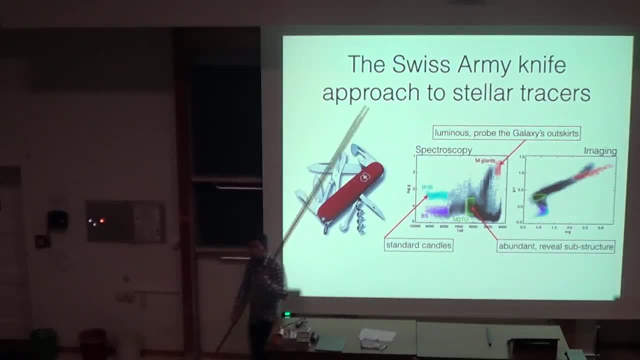 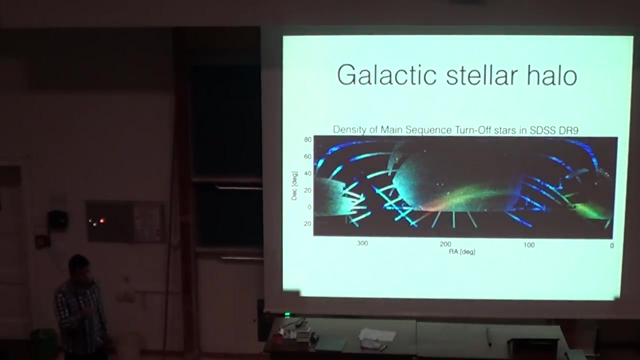 that you can pick up encyclopedial stars and blue horizontal branch stars and M-giants because they are similar. so I've shown you how the Andromeda's stellar halo looks like. that's how the Milky Way stellar halo looks like, if you use. 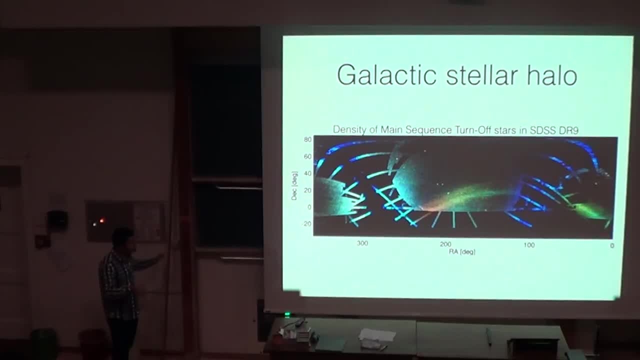 M-sequence and M-sequence terminal stars, and here on x-axis is right ascension and y-axis is declination, and what's used here is again is the stellar density, color coded according to distance. so the red stars are further away and the blue stars 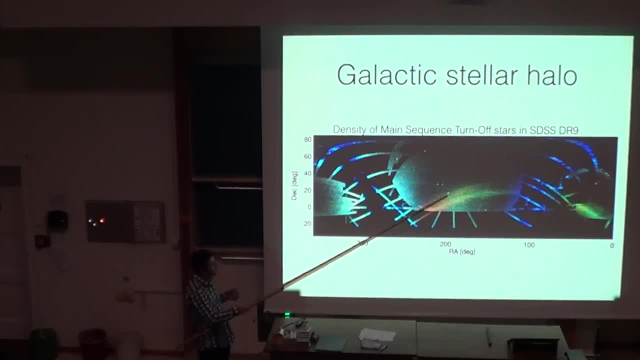 are further away, so you can see that there are clouds of stars. there are streams that are broad. this particular stream is from Sagittarius dwarf galaxy and you actually see two streams. it appears to be bifurcated. there are thinner streams like this one, yet thinner. 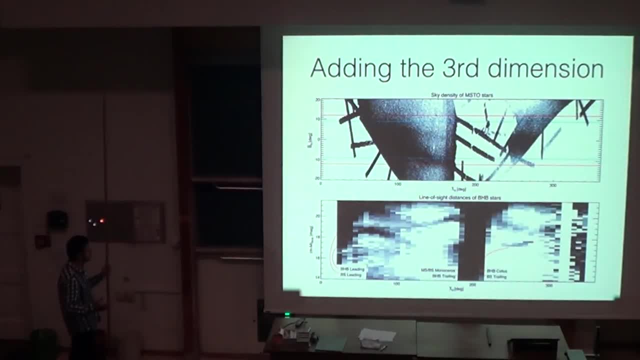 and colder streams, like the stream from the volume r5 globular cluster. so now we need to extract as much information about the phase space of these substructures as possible. so now we need to switch the tracer. so we're going from M-sequence- M-sequence. 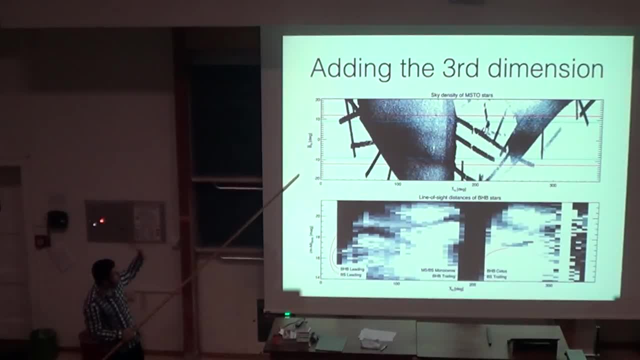 terminal stars into blue horizontal branch stars. so here's slightly different coordinate system, but it's still positions of stars on the sky so I just rotated that it's aligned with the Sagittarius stream. the panel below shows on x-axis is the distance along the stream. 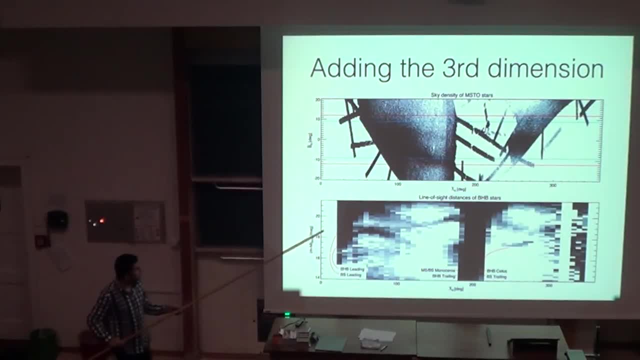 and on the y-axis is the distance along the line of sight and you can see over there. sparks here and here. these are blue horizontal branch stars that are in the stream and there are two tails that we see: leaving that is closer and trading that is further away. 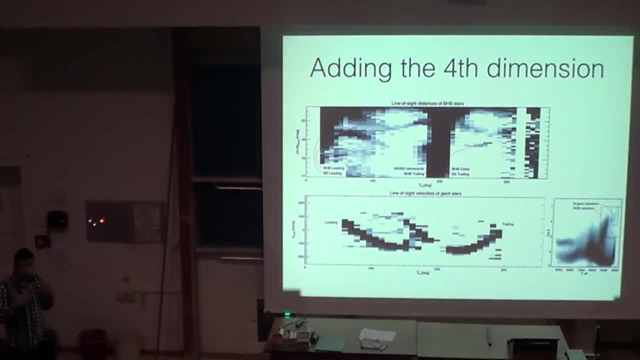 you can use k-giants and m-giants to trace the velocity track of the stream. so here I'm using the spectroscopic database and selecting a particular class of stars, and the selection box is shown on the right here and if I go again in the 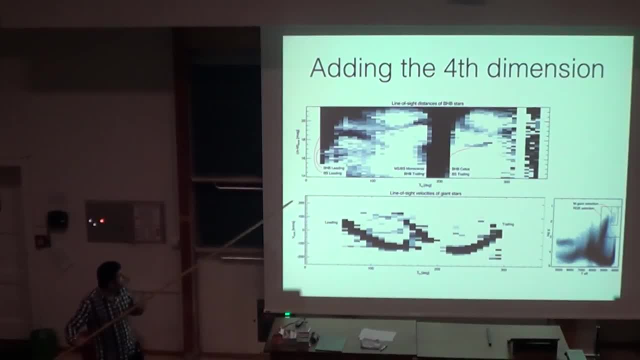 along the stream direction and plot the velocity like a cycle velocity. there are very obvious tracks responding to the leading and the trailing tail. so you can see that this particular stream has two incomplete wraps, one leading and one trailing around the galaxy. so essentially, if you remember that animation, 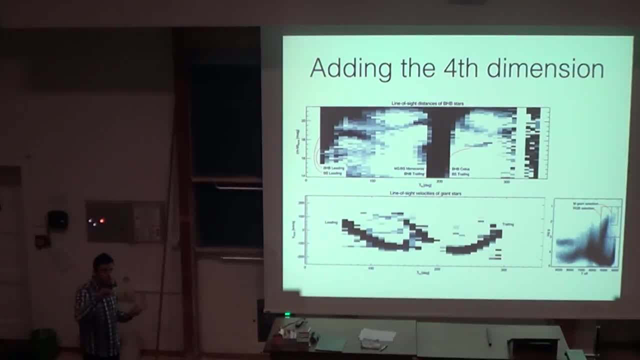 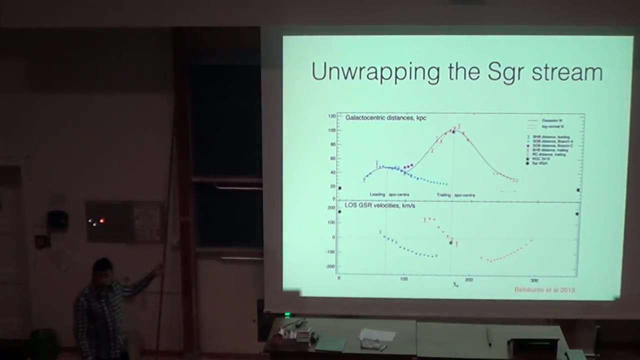 that I showed you earlier. this corresponds to two loops, two petals of the rosetta pattern that the progenitor draws in the orbital plane, and that's important if we want to now measure the properties of the galactic rotational potential. so here is the measurement of the stream. 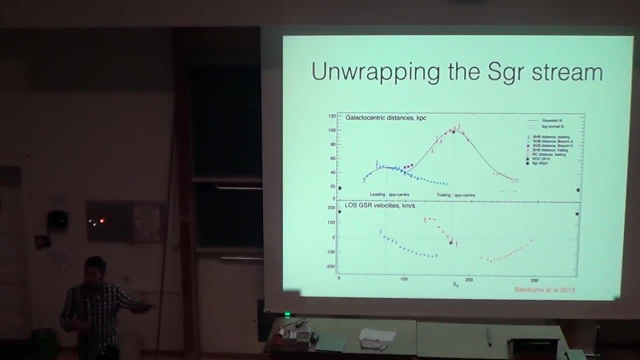 now you can see that we have two layers. so essentially we model these density plots that I showed you earlier with a background plus stream detection, and we can extract the run of distances, which is the top panel, and the run of velocities about each of the tail of the stream. 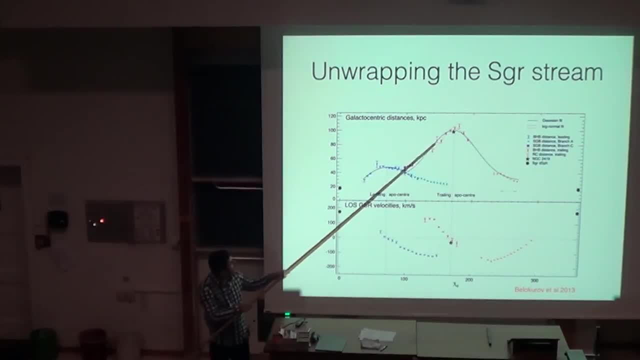 and you can see that the leading and the trailing reach upper centers, leading at around 50 and trailing at around 100 and 160 in this plane. and every time the stream reaches the upper center, the radial velocity has to go from zero and the velocities are shown here. 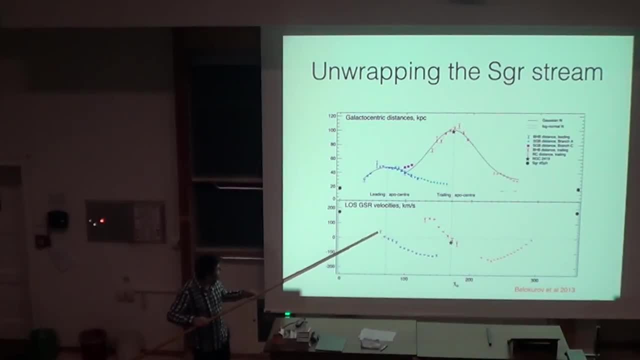 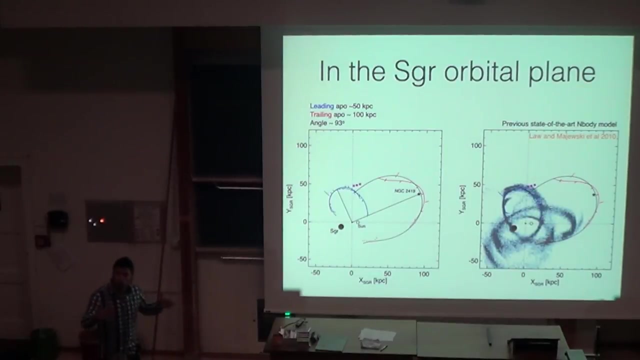 and you can see that, corresponding to each upper center, radial velocity indeed goes from zero for leading and for trailing. so the radial velocity data makes sense and is extremely useful when we want to confirm or model these streams. if I go into the orbital plane of Sagittarius, 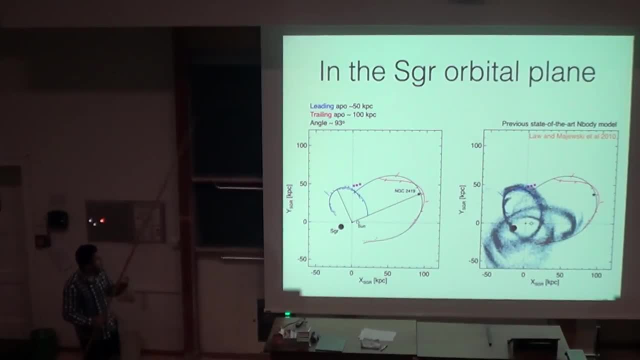 dwarf. here is how the detections that I just showed will look like. this is the galactic center. this is the sun as we are with. this is the location of the Sagittarius dwarf, and here is the leading tail and here is the trailing tail on the right. 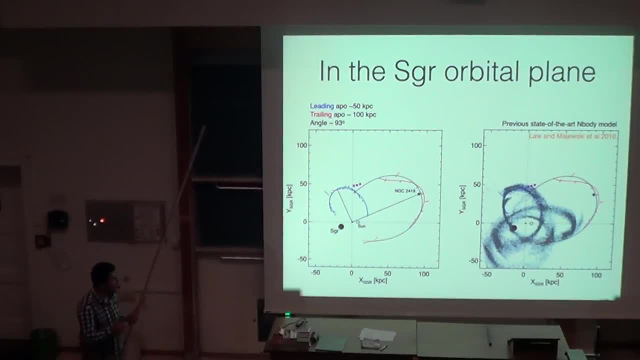 I am showing the same detections in color, but the gray scale density underneath shows one of the most representative models of the Sagittarius dwarf. so you can see that there is something that is reproduced very well in the model of disruption and something that is amaze. 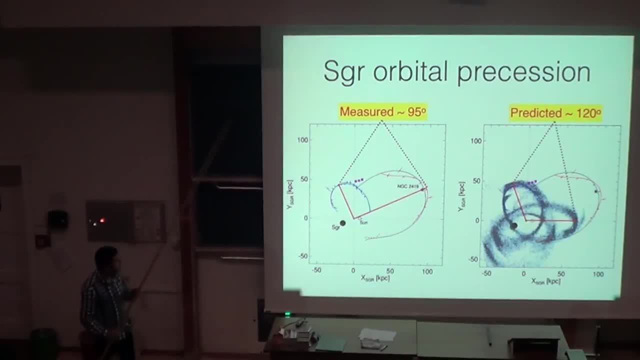 what is not really matching very well. what is matching very well is the behavior of this leading arc and the beginning of the trailing arc. what is not matching very well is the further detections of the trailing. so you can see that the in the model, in the disruption, 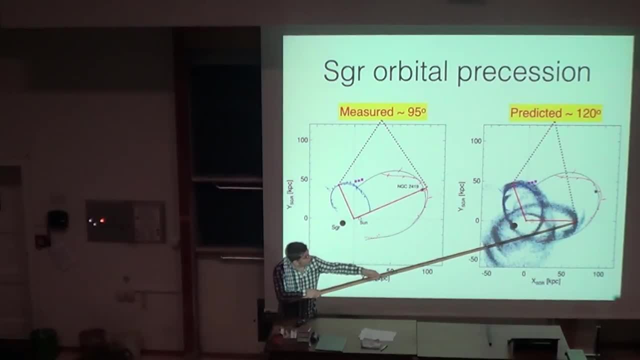 model, the trailing turns around and the upper center of the trailing stream is somewhere in the galactic disk. in the data we see that it turns around much later. the upper center is much further. so what does it mean in terms of documentary distribution? so, as I mentioned, 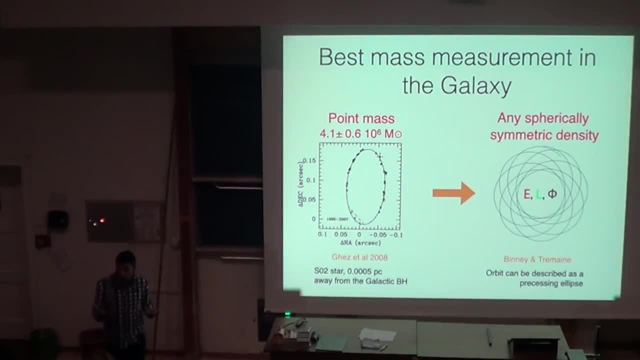 before. if we had an orbit, that should be the most straightforward way and most accurate way to infer to measure the mass distribution, and that has been proven recently with the measurement of the supermassive black hole in the center of our own galaxy. here is an orbit. 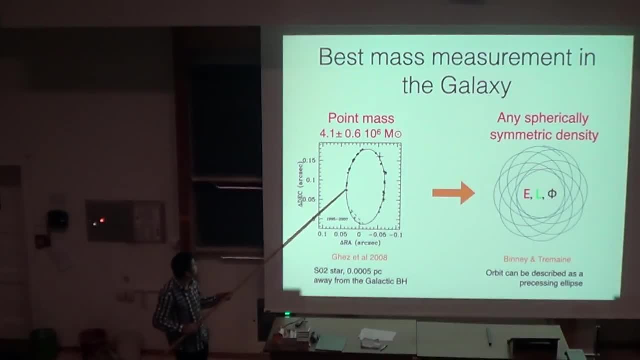 of one particular star that took slightly more than 10 years to almost complete. and this orbit looks like a Keplerian ellipse and it gives you a mass measurement which has an error of order of 10% and, of course, this orbit has a size that is. 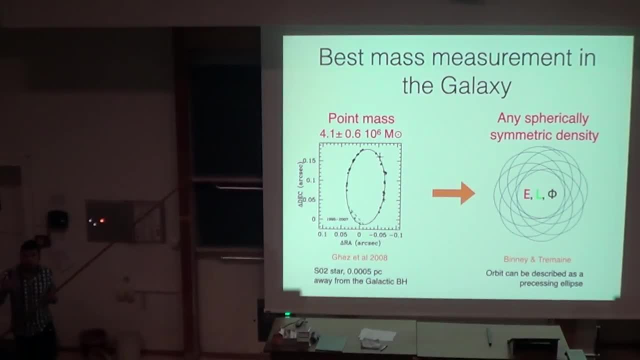 10,000 times smaller than a parsec. now we want to do the same experiment, but at distances that are 100 kiloparsecs. so many, many, many orders of magnitude larger distances, encompassing a huge amount of mass, most of which is in dark matter. 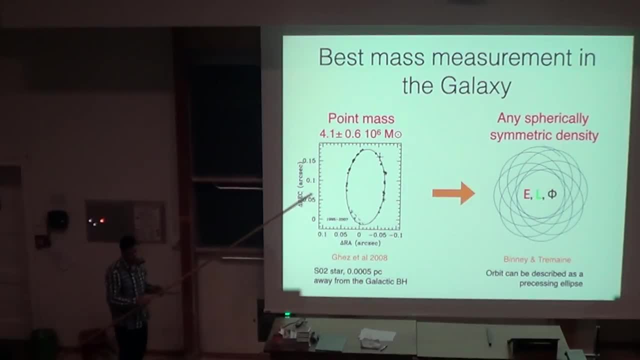 in the galaxy. so this particular potential is really simple. it's dominated by the supermassive black hole. so it's a point: mass potential. that's why the orbit is the ellipse, or in other words the orbit closes onto itself. so if the mass distribution is still 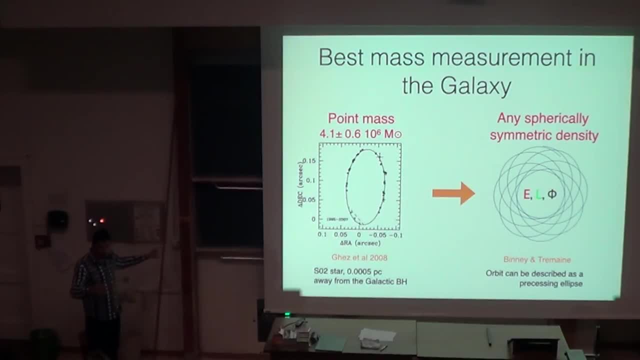 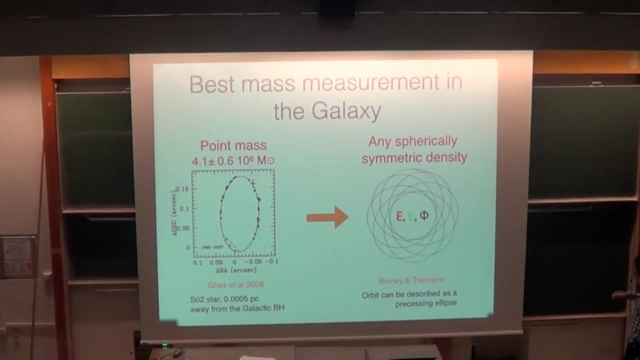 statically symmetric but is distributed along the radius, so it's not concentrated with one particular point. then the mass will start to precess. this ellipse will start to precess, and you saw this already in the little animation that I showed you, and this simple intuition can be. 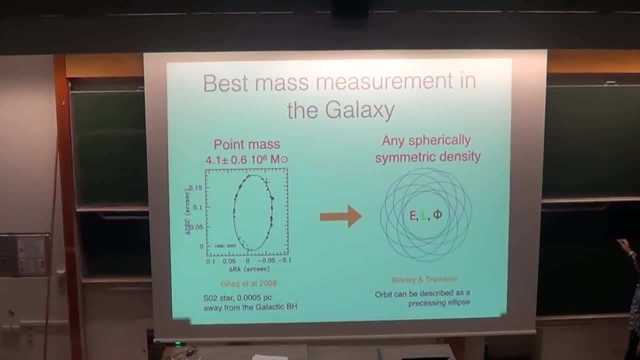 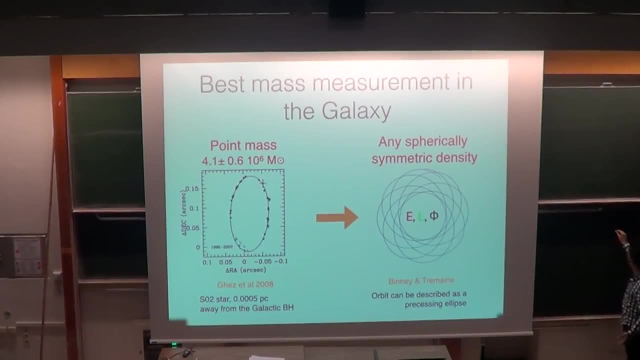 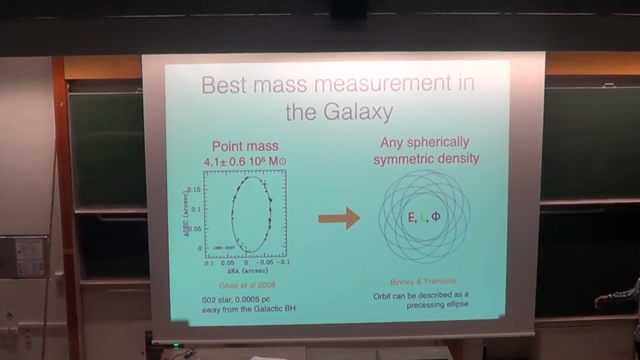 so imagine you have a center of the galaxy and a satellite that falls into it and somewhere around the epicenter it sees all the mass that is that reaches to pericenter, because the mass is regularly distributed. suddenly what it realizes is that its velocity is too fast. 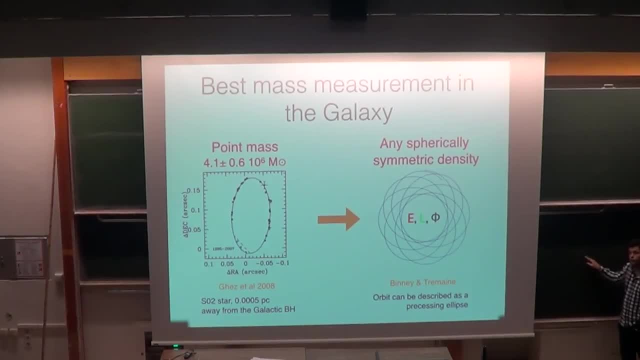 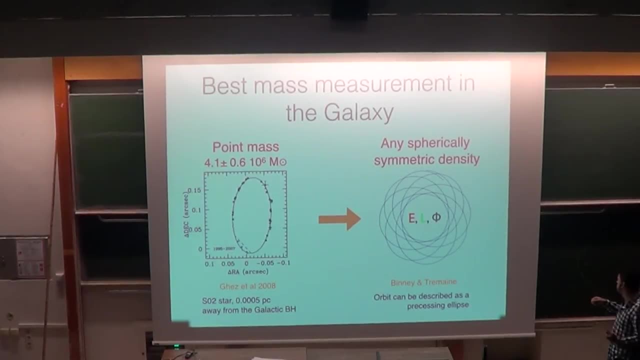 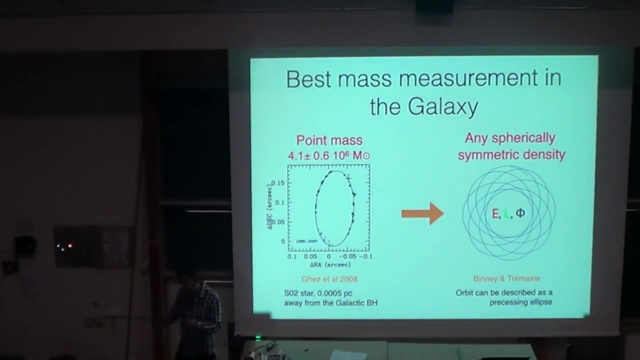 to the amount of mass that is inside the pericenter, so it overshoots. so that's why the orbit starts to precess. and, of course, if you knew the size of the orbit and its eccentricity, which essentially is governed by energy and angular momentum, 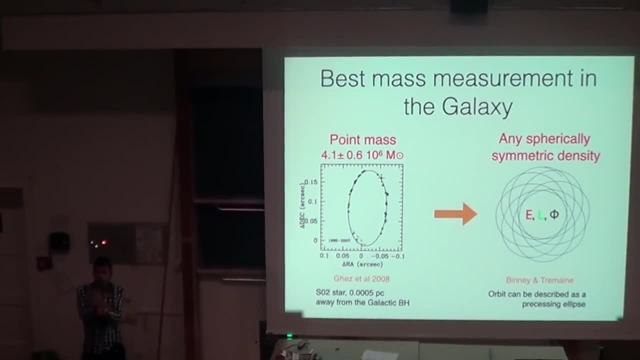 of the orbit. the remaining factor that governs the opening angle between the petals, between the successive pericentric and apocentric passages, is the gravitational potential. because we made the gravitational potential spherically symmetric, the only thing that is left interesting in it is the rate. at which the density of the density now controls the opening of the petals. so if you put all the mass in the center, so you make this slope extremely steep. the orbit will close onto itself. if you redistribute the mass as flat as you can, you make a little. 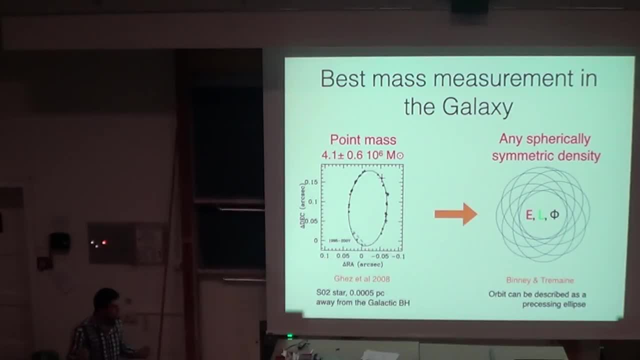 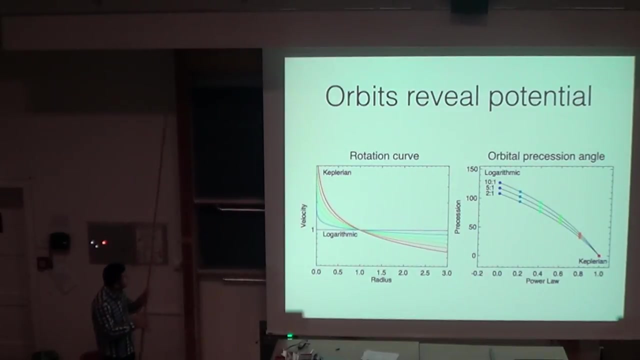 rifting angle right, then you open the petals by 120 degrees approximately. so if you can measure the density distribution of dark matter in the galaxy, and this particular polar illustrates exactly that. so here are different potentials. the potential here is a power law and this is the 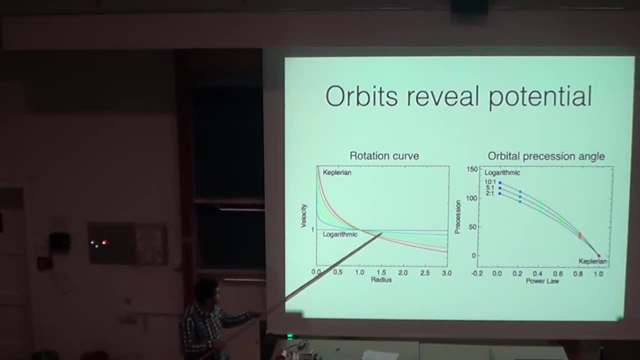 corresponding circular velocity curve, right rotation curve. so here is what it is, with a flat rotation curve and a Keplerian curve and everything in between. so all that's changing here to literally thick. and here is the precession angle, so the opening angle between two successive petals. 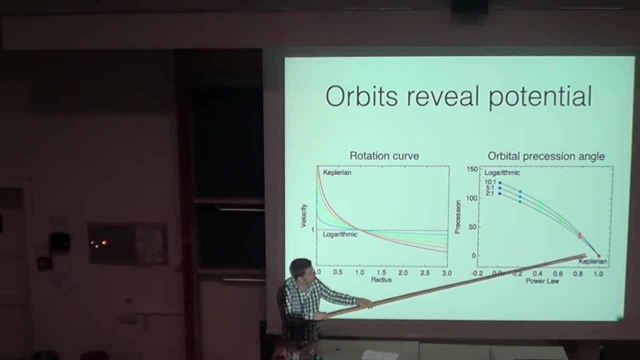 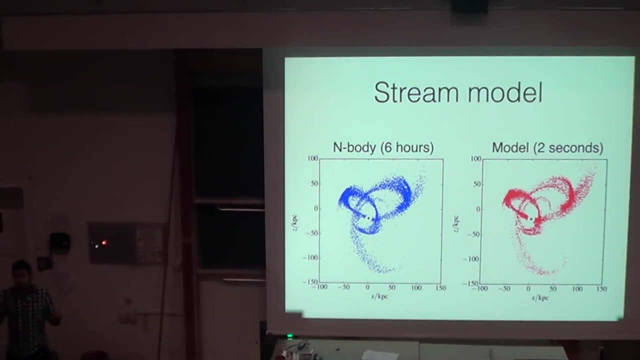 of the orbit and you can see as you make the mass distribution flatter and flatter, the angle increases. so if streams were orbits, we could just use that plot. read the, the, the, the orbits. you can make a stream if you run a body code and you 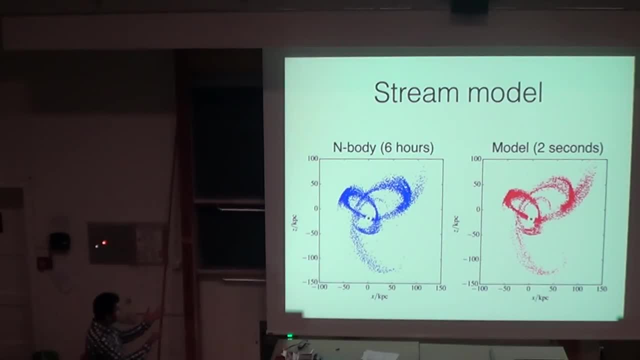 disrupt a progenitor and you produce a stream that looks like this on the left. so this is, in the orbital plane, the distribution of debris from a progenitor which is now here, and this takes quite a long time because you are calculating the forces between all particles that you put inside the progenitor. You can make it much faster if you avoid calculating. 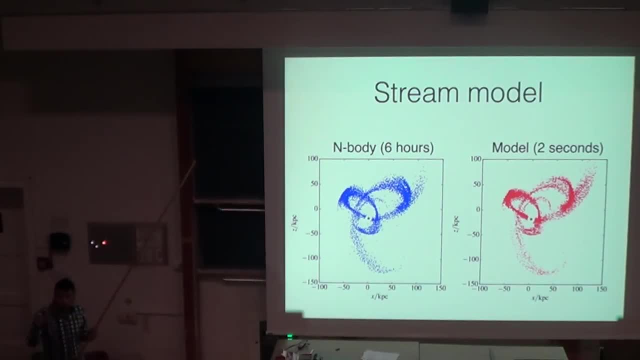 the forces between the particles and if you give them particularly initial conditions- And I already showed you what initial conditions you need to give particles if you want to produce stellar streams- You start them at Lagrange points, And that's exactly what we do here. So this is our model that mimics this at-module simulation And of course it's. 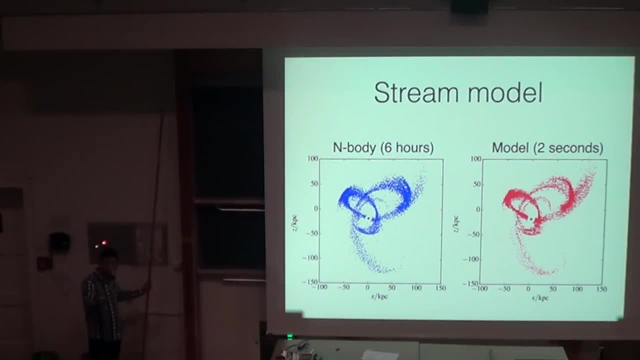 much faster because we're not calculating the gravity between the particles and we're given very specific initial conditions releasing these particles at Lagrange points. So in essence, we are solving constraint-free body problems where the particles are orbiting real-to-real potential in the presence of perturber, which is the progenitor from which 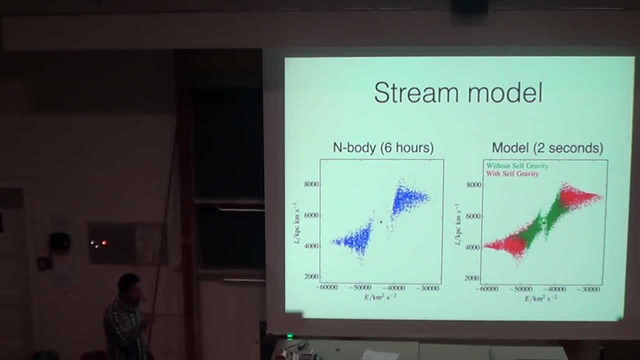 they're left And it turns out that the gravity of the progenitor is extremely important. So here's the energy. So here's the energy for this simulation in the energy and angular momentum space. So these are the particles that left the progenitor and now form the trailing and the leading. 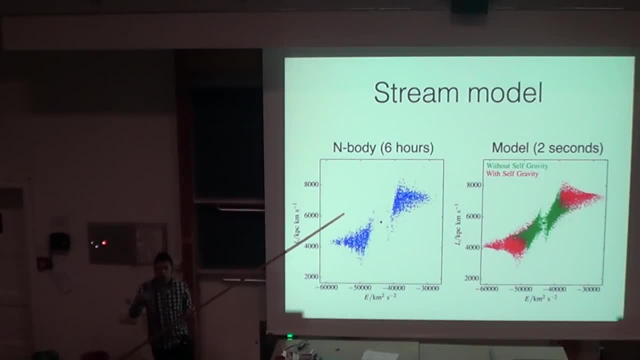 debris. So now, if we just release the particles at Lagrange points without the gravity of the progenitor, that's what we get. These are the green distributions. So if we turn the gravity of the progenitor on suddenly, we get back more or less correct distribution. 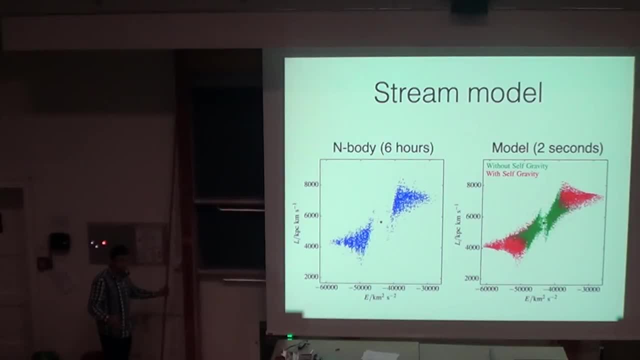 of the phase space coordinates of our particles. So the progenitor is important and I think I know why, but I don't want to waste my time explaining it now. But if you want to know, I will try to explain it later. So now we have an extremely fast model that produces 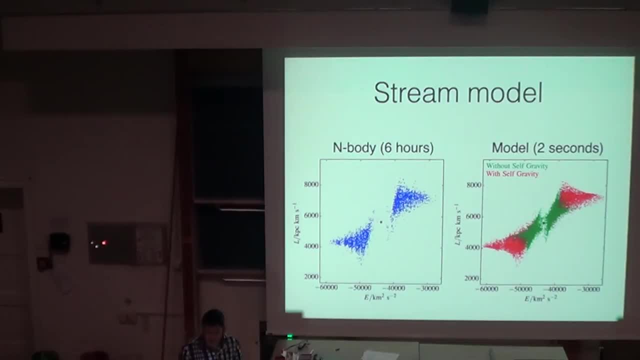 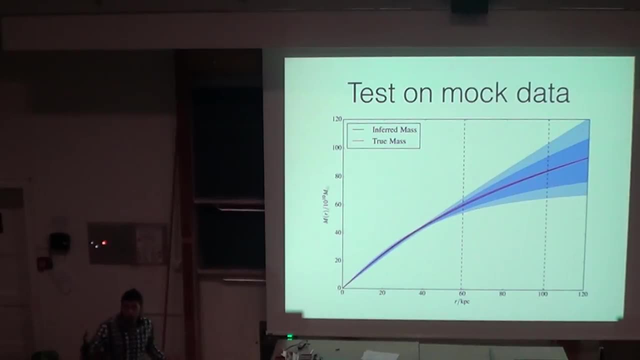 very good looking, correctly looking streams. So we can now try to model the Sagittarius stream data that I showed you earlier. But before we do that we test our model on mock data, And here the red curve is the true cumulative mass distribution as a function. 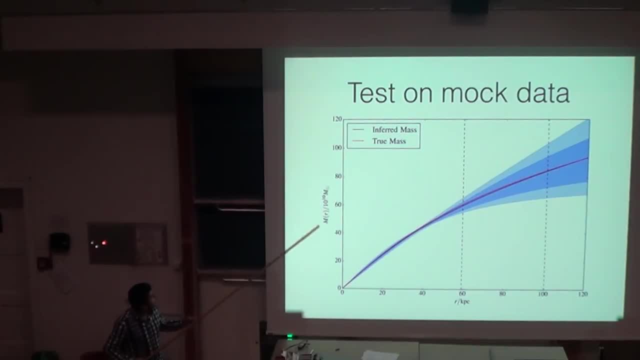 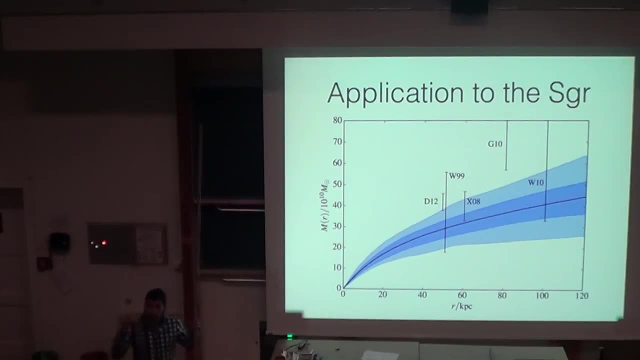 of the radius in the mock data set And our inferred mass is the black curve and 1 and 2 sigma contours are shown in different shades of blue. When we apply the same method to Sagittarius stream, that's what we get. This is our inferred cumulative mass, with 1 and 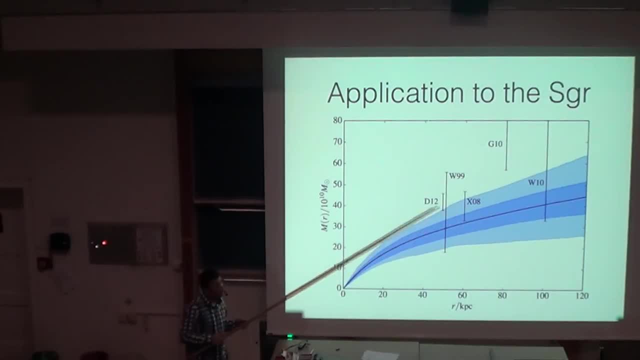 2 sigma contours, And here are previous measurements that mostly employ genes modeling. You can see that we go typically through the lower parts of this error bar, which is interesting, and also that our 1 sigma error bar is typically smaller than our previous measurements. So 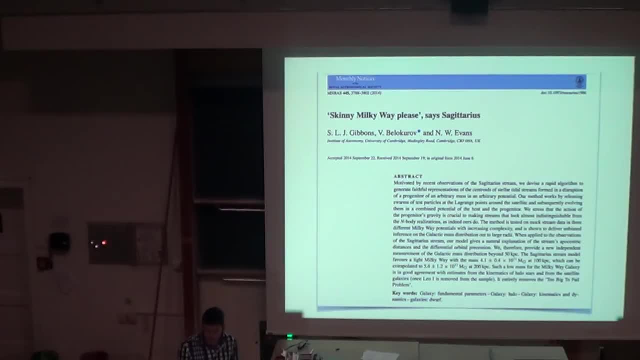 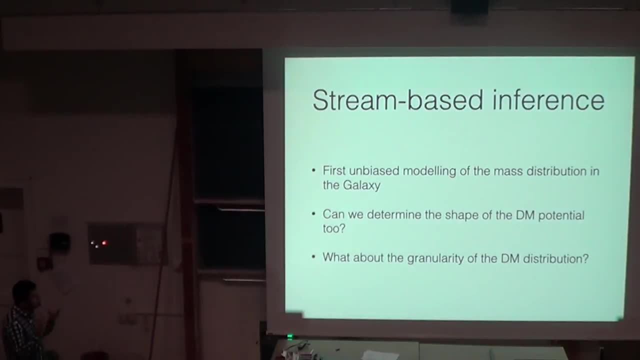 this work is described in a paper led by Simon Gibbons, who is a PhD student at Cambridge. So what we've managed to do is we've produced a new modeling tool that allows us to produce unbiased measurements of the mass distribution in the galaxy. We can hope to use this to 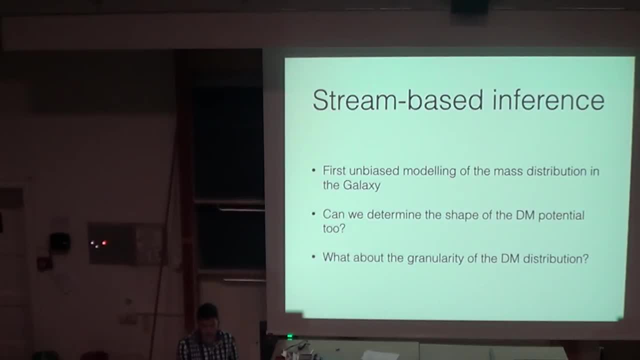 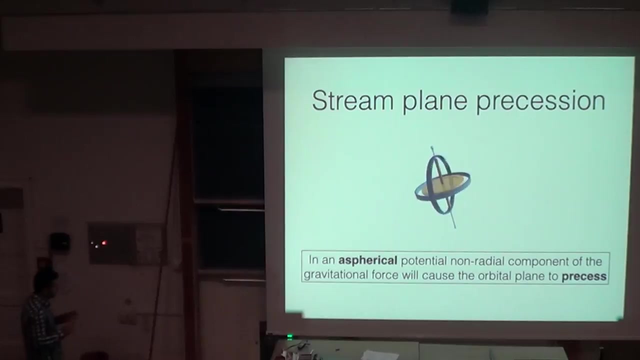 also determine the shape of the dark matter potential And we have ideas of how to use similar techniques to measure the dark matter mass function. To understand the shape of the galactic dark matter halo, we now need to look at the precession of the orbital plane. 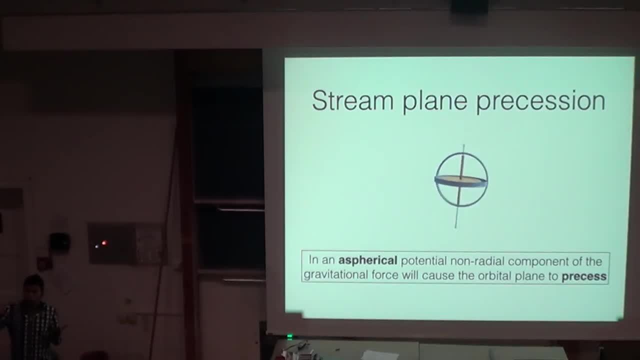 of the galaxy. So what I talked to you about before was the precession of the upper center, so-called obsidial precession, So the precession of the ellipse due to a distribution of matter along the radial direction in the host. So the orbit doesn't close onto itself and it 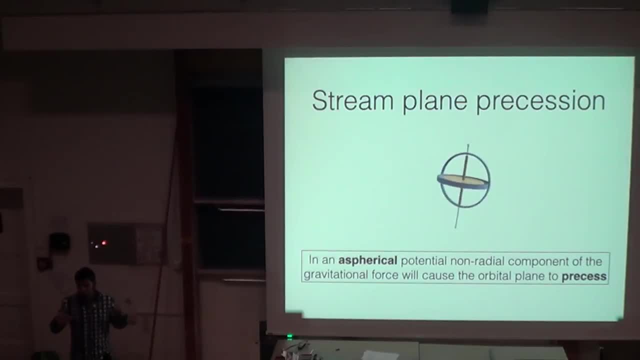 rotates in the orbital plane. Now, if the dark matter distribution is a spherical, there will be torques acting on the orbital plane, So the plane itself will start to precess. So the orbit will precess inside the plane and the plane itself will start to precess. 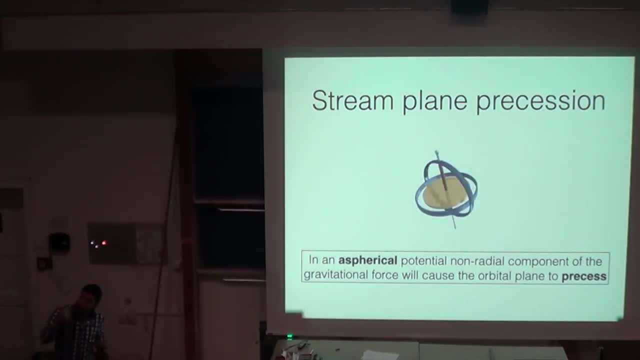 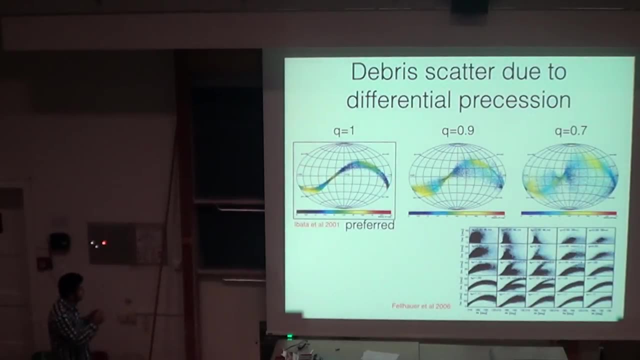 So if we can measure the precession of the plane, we will determine how aspherical the dark matter distribution is, And this idea is not new. For example, Pate et al already showed that if you make the dark matter halo, very aspherical streams like Sagittarius. 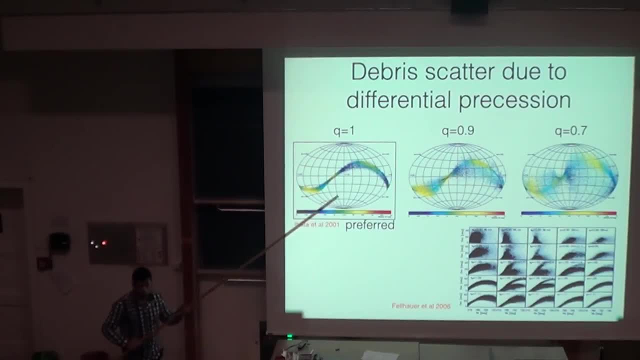 this is a spherical case- will start to spray around the galaxy due to the dark matter distribution. So they dialed down Q, which is the flattening, so they made it very flattened or blade, and very quickly the stream exploded. I'm not actually sure if this is physical or not. 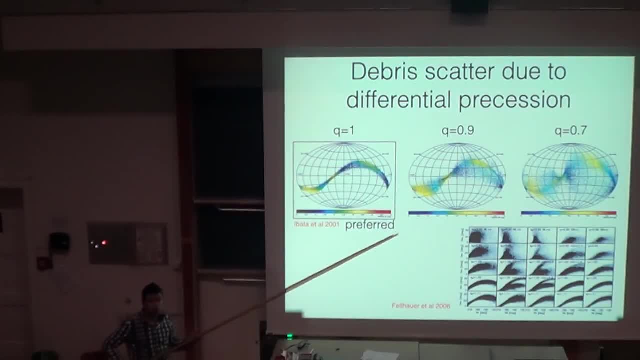 So a similar idea was explored by Volkowartov, which also showed that to produce a stream like Sagittarius, you need a potential that is very close to spherical. But that's not what we're doing. We're not measuring dark matter spraying around the galaxy. We're 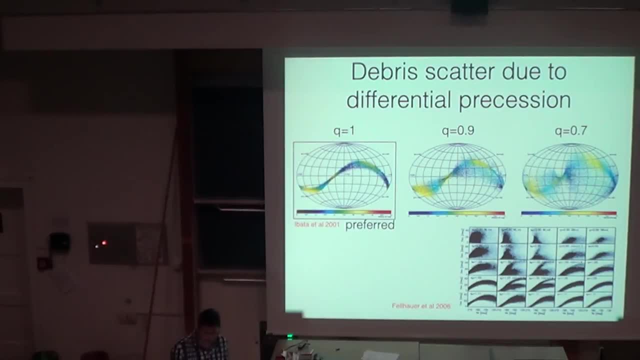 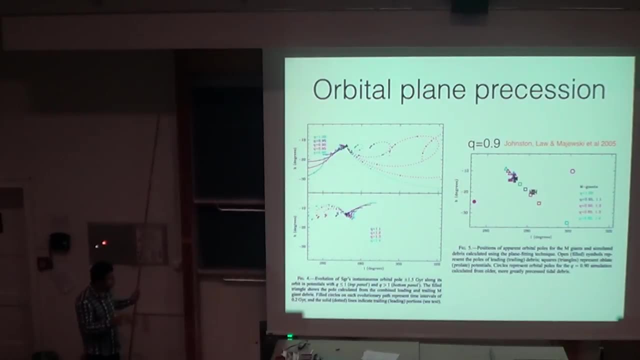 measuring the level of spraying that is due to differential precession of stars in the stream. What we're more interested in is the idea highlighted by Katherine Johnston is actually measuring the plane of the debris and its evolution as you step through the stream, And so here is the coordinates of the pole of the orbital plane, or basically, 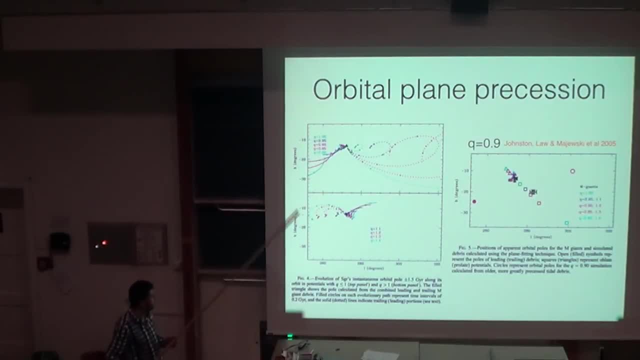 where the angular momentum of the plane is showing on the sky. So these are L and B galaxy spherical coordinates. Here are the orbits, and this potential is flattened or different amounts. So here is the flattening, And what we're showing is that, depending on 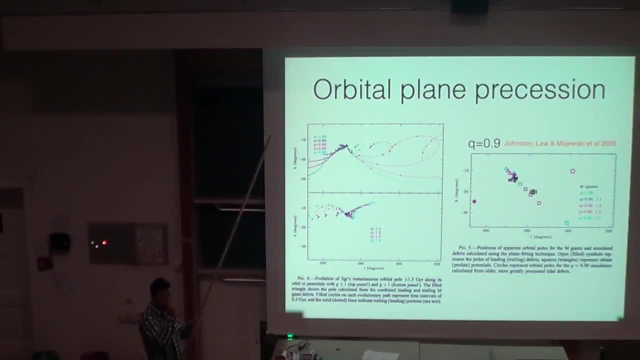 the flattening, the orbital pole, the angular momentum vector, will draw these loops on the sky And this path, this loop on the side, depends on the flattening. So of course, with the stream, you're not measuring the orbit, but you're measuring the orbital plane. you're. 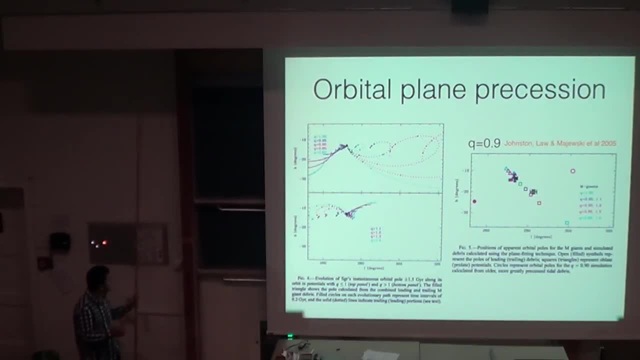 measuring the degree plane. So they tried to do this. They could measure the plane in two, the exact degree plane, in two positions along the stream. So that's what was known in 2005.. And their measurements for the leading and trailing parts of the Sagittarius stream. 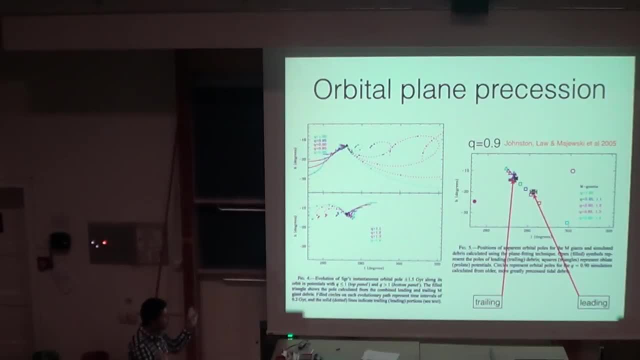 indicated that those orbital plane, the degree plane, are quite different from each other of order 10 degrees or so, And they concluded that the flattening of the orbital plane is the same as the flattening of the potential. It should be a 4.9, so it's an ablate quite 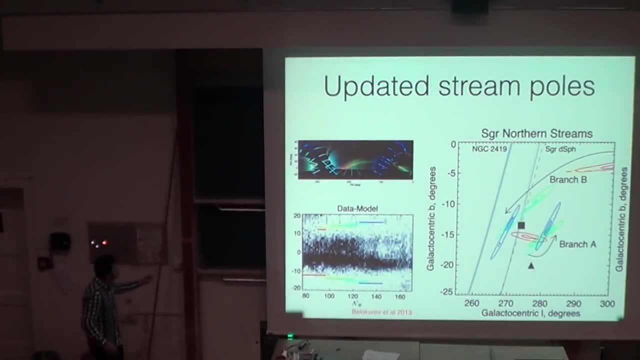 flattened potential. We have much better data now so we can concentrate on the best studied part of the Sagittarius stream around here. So here I get rid of the background, this Pelletier background that is well mixed, and only have the orbit density due to the streams. 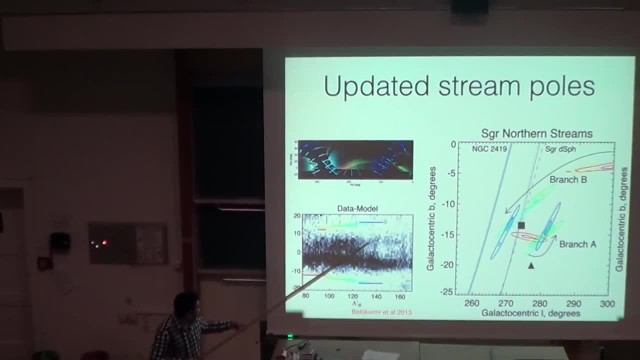 And there are two streams, one right and one slightly thinker, Because they have blue horizontal branches, distances, they have enough fluid information And I can feed planes through the galactic center, because orbital planes have to go through the galactic center. And 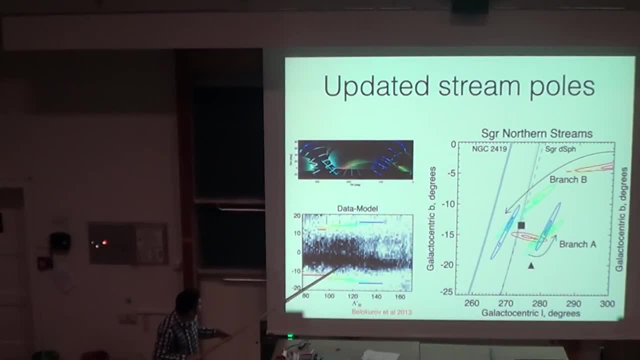 they jump off the stream, And so I split it into red, yellow, green and a change of blue pieces, And for each I plot the orbital pole or the plane pole on the sky. So this is again galactic centric L and B And that's how the pole evolves as you step through the 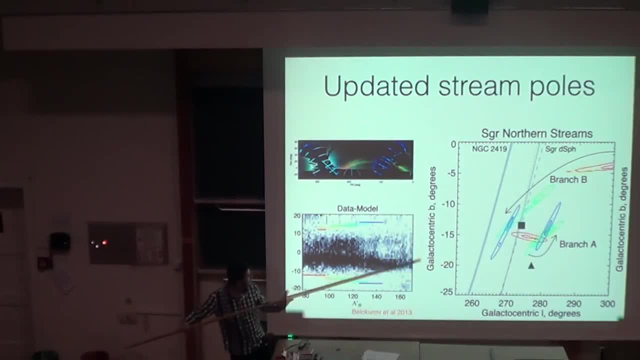 stream, For the bright, branch A, for this blue stream and for the faint, so the upper stream. as you go, starting on the left and going to the right, evolution is very different. So this is somewhat bizarre because these two streams seem to indicate very different. 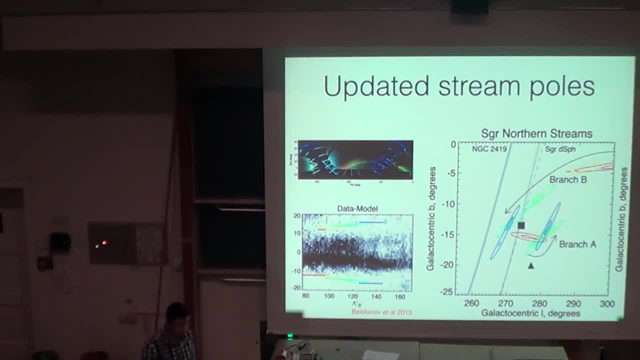 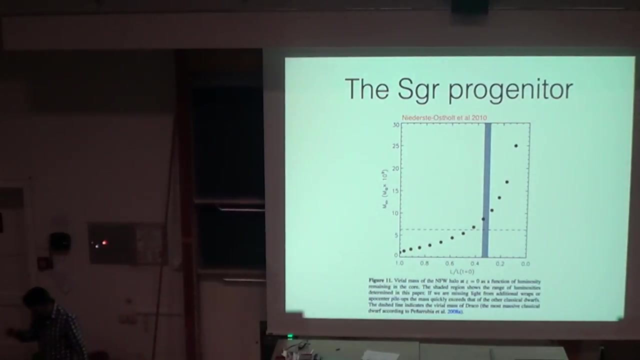 evolution in the same rotation of potential. So the sense of precession is different there, The precession happens in a different direction And the amount of precession is different there. What is important when we try to interpret this is to remember what Sagittarius dwarf could have been before it fell into the Milky Way. We think that Sagittarius dwarf was the third most massive dwarf galaxy around the Milky Way, after the Large Magellanic Cloud and Small Magellanic Cloud, And we think so because we've calculated the amount of 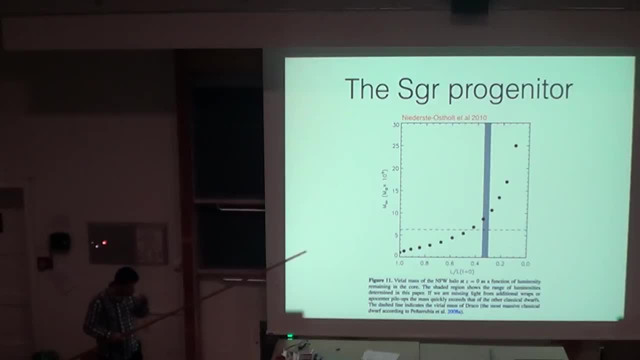 luminosity in the stream and put it back in the projection of the Milky Way, And we have a limit on the total luminosity of the projector before it fell by collecting all the stars and the streams. So this is the luminosity on the x-axis and the mass on the 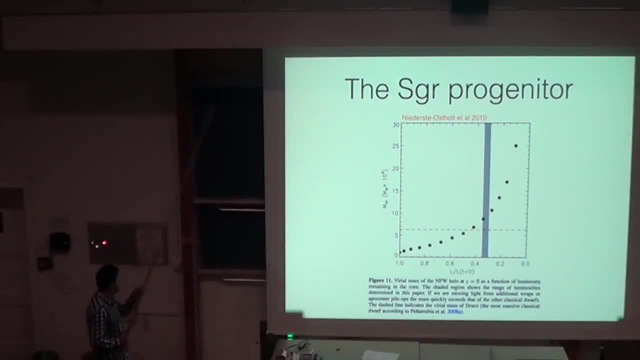 y-axis using the dwarf galaxy models of the Milky Way. So, given the luminosity of the order of 10 to the 8 solar, we get an order of 10 to the 9 to 10 to the 10 solar masses in the projector before it fell. 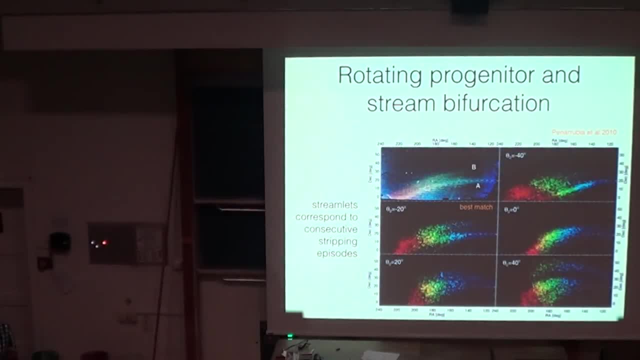 And given such high mass for the dwarf galaxy, it is likely that it was rotating more irregular. If the dwarf was rotating as it infilled into the Milky Way galaxy, something interesting can happen. Every time the disk dwarf goes through the pericenter it shows a different 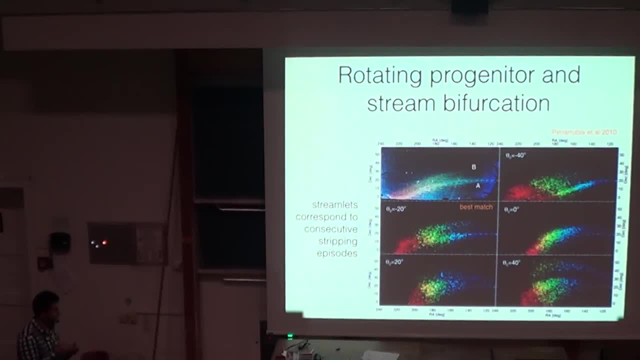 part of its disk to the galactic center And so the angular momentum in the disk, which will add to the angular momentum of debris different amounts of it will, So the sprays of debris that leave through Lagrange 1 and Lagrange 2 will have slightly different angular 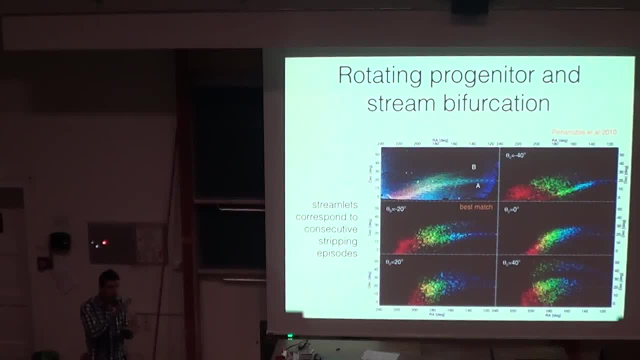 momentum and energy. So you can split streams into multiple streamlets depending on the orientation of the disk in worth with respect to its orbital plane, And that's what Park and Yerubbe shows here. These are different orientations, misalignment angles between the orbital plane and the disk. 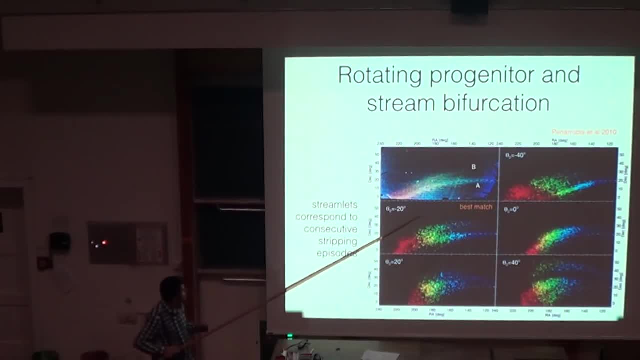 disk to progenitor. So 40,, 0,, 20,, 20 in a different direction and plus 40. You can see that when the two planes are aligned completely, this stream looks like the ordinary stream from a pressure-supported dwarf galaxy. But when you start to misalign them, you create. 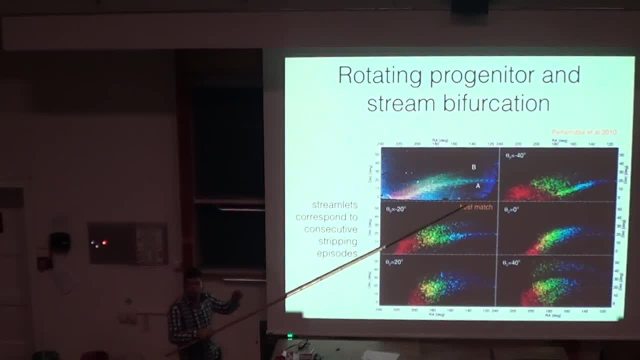 these sprays of the debris that go off the orbital plane of the progenitor- And that's something of the progenitor of the progenitor in different directions, And you create these bifurcations quite naturally. And so, in the Yerubbe 2010,, the conclusion was that a progenitor 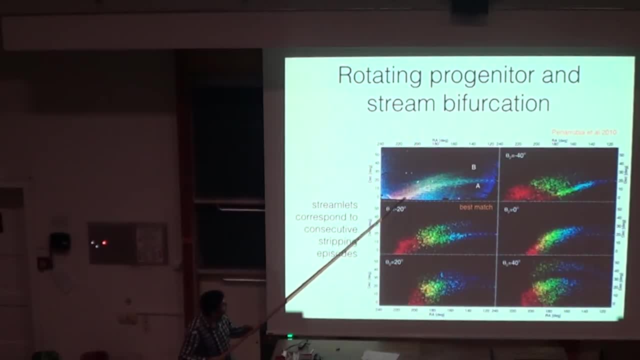 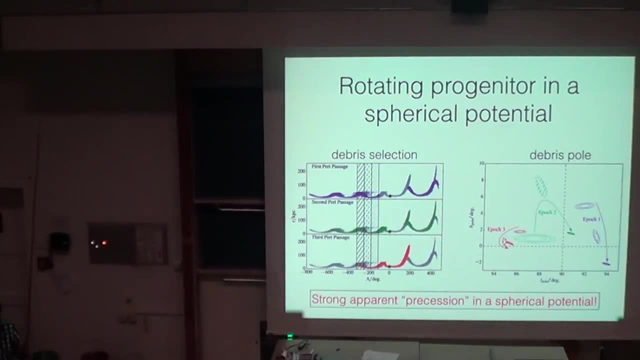 that's misaligned by 20 degrees with respect to its orbit reproduces best their simulations. But something interesting happens when you send a rotation progenitor in a spherical rotational potential. So in a spherical rotational potential there are no torques acting on the stream particles. 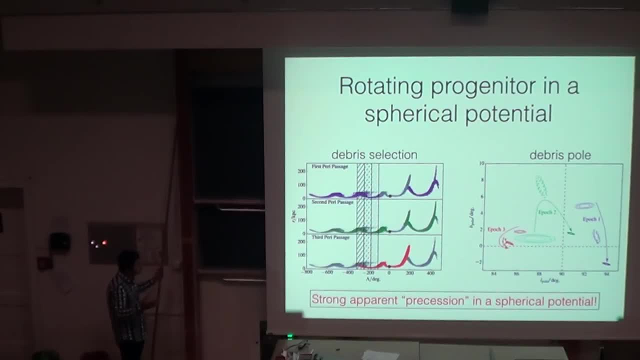 on the stream stars, so they shouldn't present. However, in this experiment we did exactly that. We sent the rotating dwarf in the spherical potential it disrupted, the stream is produced and there are debris that are sprayed out of the progenitor after the first periscopic 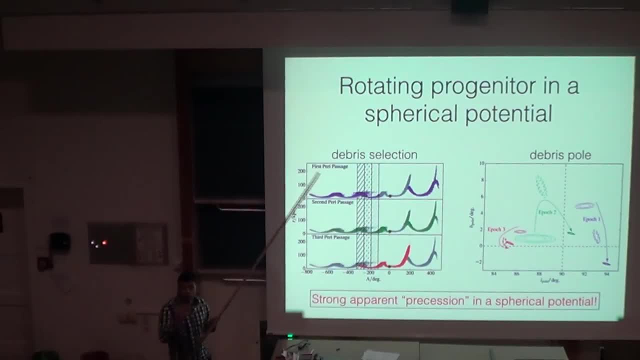 passage second and the third. And when we look at the evolution of the orbital plane- they're shown here. This is the pole of the plane, or the momentum. They seem to evolve in very different ways and by different amounts, even though the potential is spherical. so 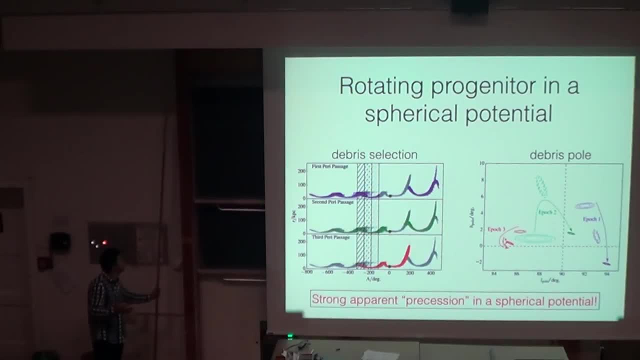 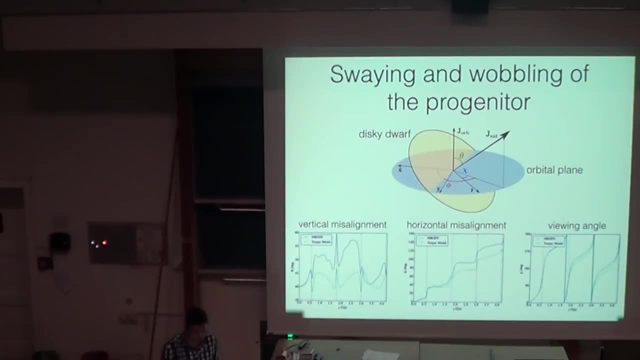 there are no torques acting on these orbital planes, on the orbital planes of these stars. So that's somewhat surprising, but it's not very surprising if you remember that, while there are no torques acting on the orbital planes of the streams, there are torques acting 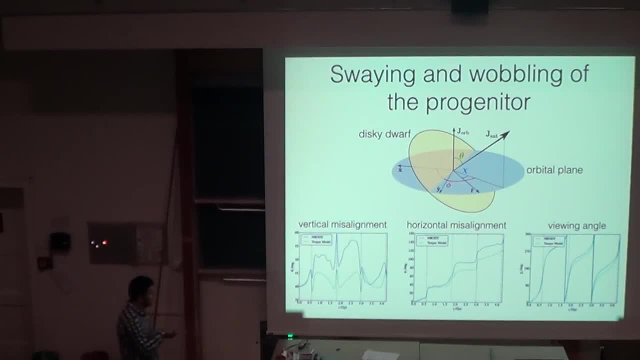 on the progenitor itself And the progenitor itself is precessing. so the disk dwarf, the small dwarf galaxy that is rotating and stripping as it rotates around the Milky Way as well, it's actually precessing under the torques from the Milky Way because it shows different. 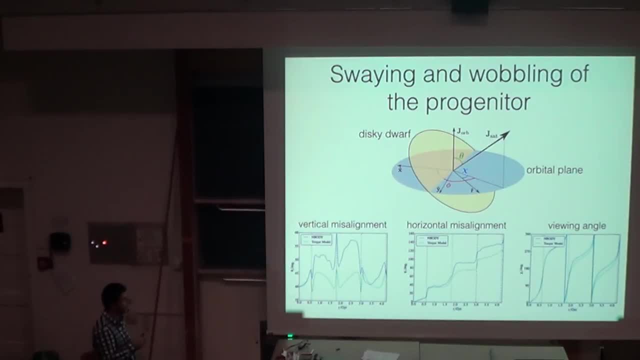 parts of its disk to the Milky Way galaxy, So if it's misaligned with its orbital plane. So to understand this better, here is the orbital plane of the dwarf, Here is the orbital plane of stars in the dwarf itself. So this angle phi is the horizontal or in-orbital plane projection of the angular. 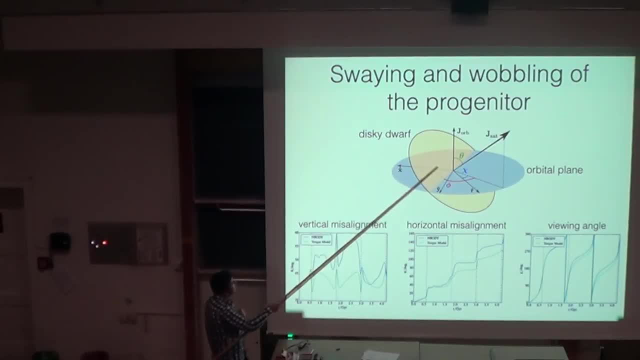 momentum of the disk And the angle theta is the vertical component of the misalignment between the two angular momentum vectors And you can see that the phi is evolving with time And it goes through these very sharp evolutions every time the progenitor goes around pericenter, So it's precessing. 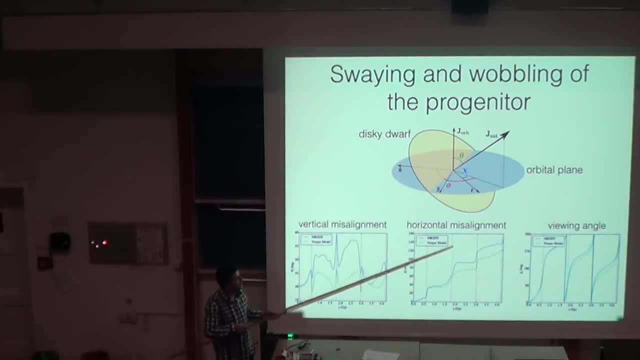 slowly, then very fast, and slowly again, and then very fast again. So, because this happens, the debris configuration- Every time the stripping happens it will be slightly different. So the stars will be sprayed with slightly different angles with respect to the orbital plane. with the original. 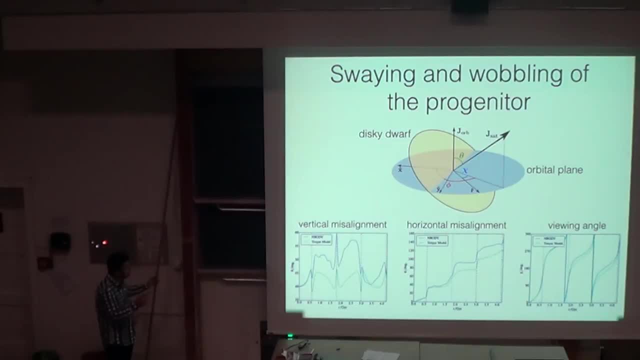 orbital plane. But what is also curious, what happens as well, is the vertical component of the misalignment. this angle, theta, also goes through a dramatic evolution around the pericenter. So our initial misalignment was 40. And it evolves. 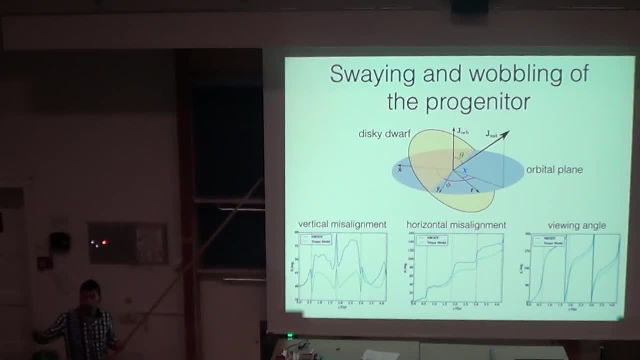 And it evolves by an order of 20 degrees along the orbit. So not only this disk is precessing as it orbits the Milky Way, it also wobbles every time it goes through the pericenter. And that's again because the orbit of the progenitor here is quite eccentric. So the arc 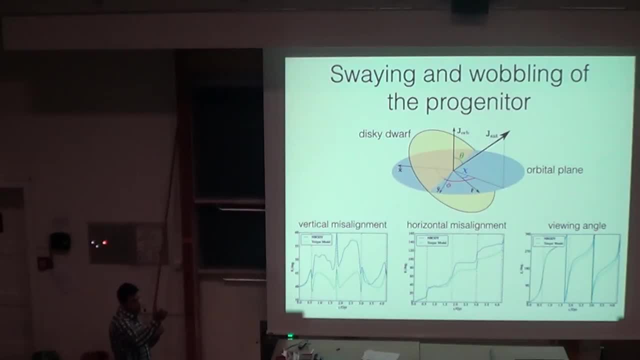 around the pericenter that covers more than 180 degrees is covered very quickly, And so the disk of the dwarf sees the pull of the galaxy on one side and then on the other side in a short period of time. So it's torqued in one direction and then it rotates. 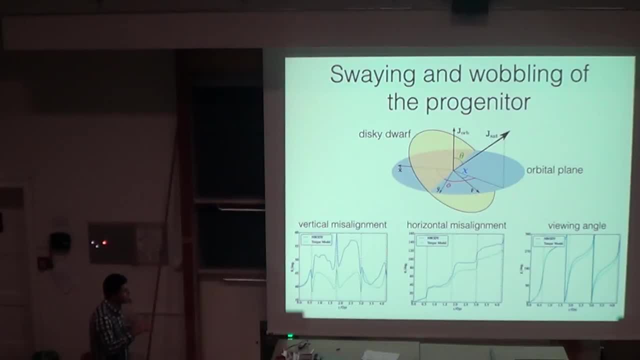 and torqued in the other direction. So it goes through this wobble. So if you want to model this, you could, Because you know the gravitational potential, so you know the force and you can write down the torque, and that's what we try to do. 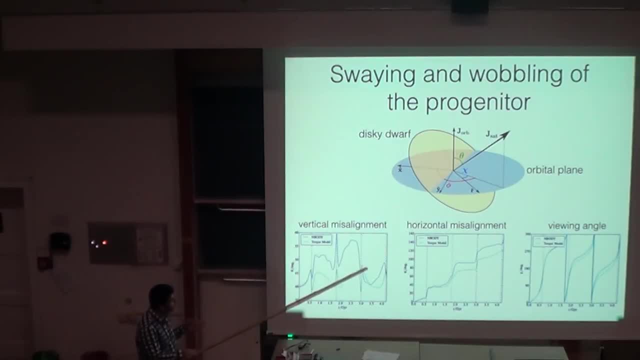 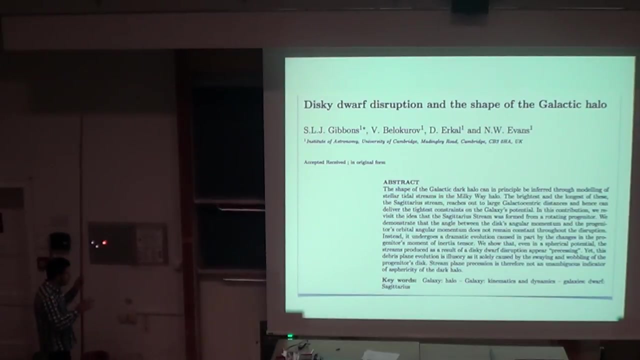 And that's the green line and it's compared to the blue line which is measured from the at-body simulation, And you can see that you start very well and then the two lines decouple, So your model breaks. And why it breaks is because the long-infinition tensor of the dwarf evolves away from the 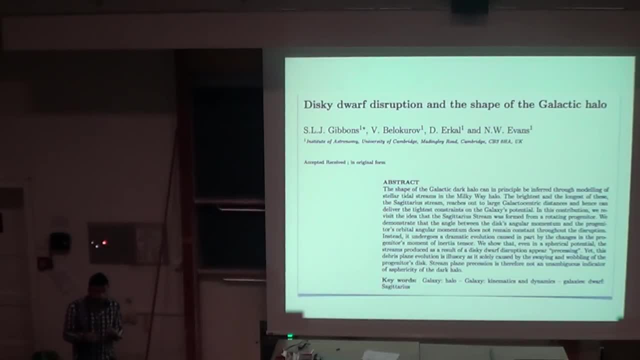 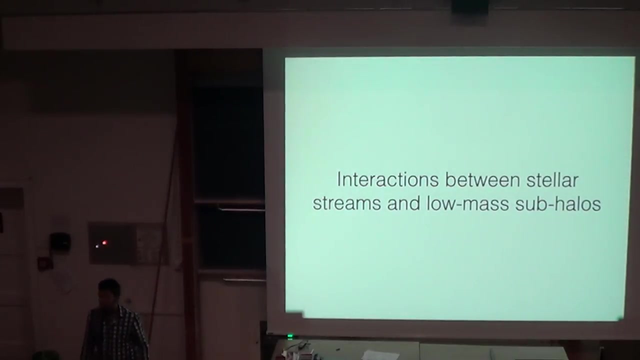 configuration in which it started, And it's a known effect. It's known as tidal stirring. So the disky dwarf is destroyed and it's slowly turning into a dwarf-spheroidal galaxy. And if I have five or something, oh, leave me alone. 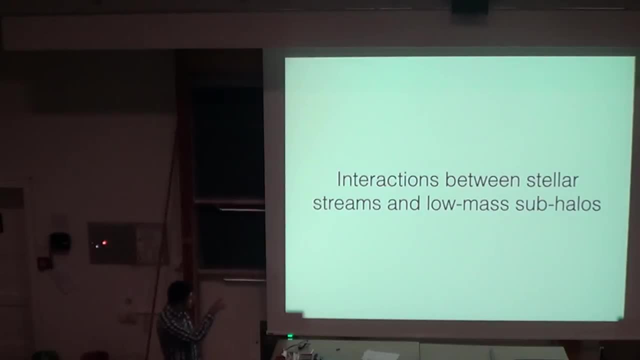 How much energy do you guys have left? So this is a final topic and I promise I'll make it very short, But I think it's very exciting Because it's the question that everyone that is into this subject wants to have an answer. 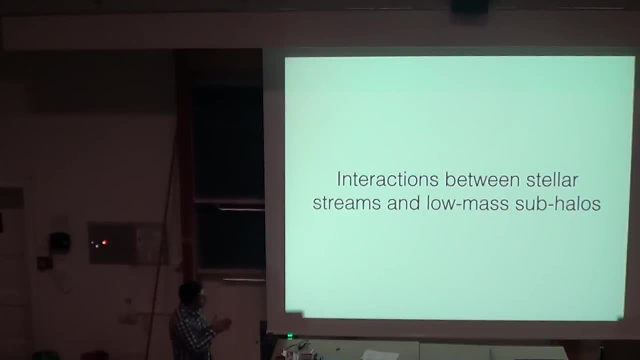 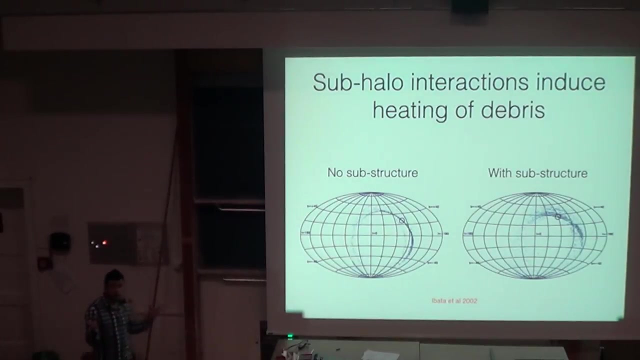 to How low is the mass of the smallest dark matter sub-halo. And here's the idea that, again, has been around for some time: If you have a stellar stream and you have these small mass particles, these sub-halos. 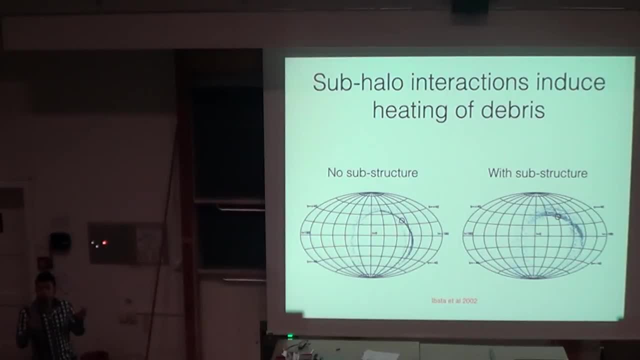 that are risen around the galaxy, they will start to hit the stream, They will puff it up. And so here is the paper by Ibahter in 2002.. It produced a stellar stream by disrupting globular cluster And it looks pretty cold and culminated. 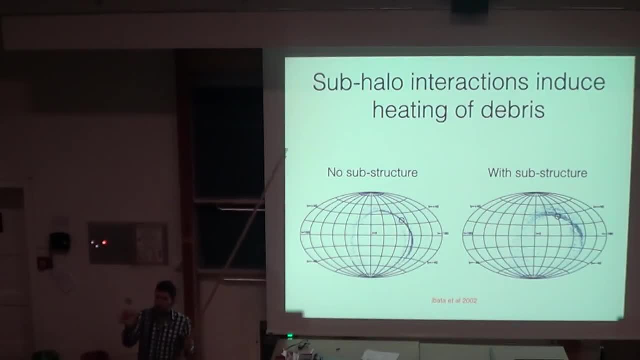 And then they redone the simulation, but they also injected small sub-halos with mass of 4 to the 10 to the 6 solar masses that are now flying around and are hitting stream particles. And you can see what happens: The whole stream is broadened. 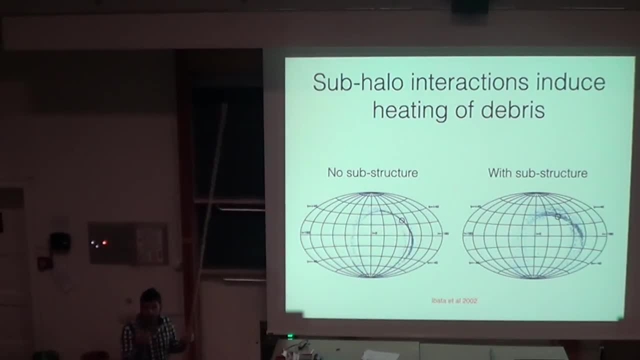 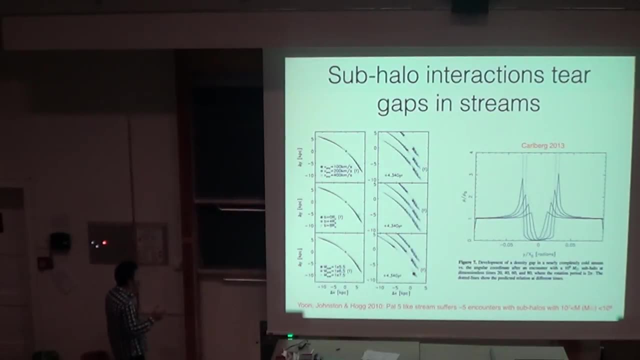 It's dispersed on the sky, So they hit the stream And this effect should be observable. However, there is much more dramatic effect that can be seen and potentially used to measure even masses and properties of data and sub-halos. When the sub-halo flies by the stream, it can tear a gap in the stream. 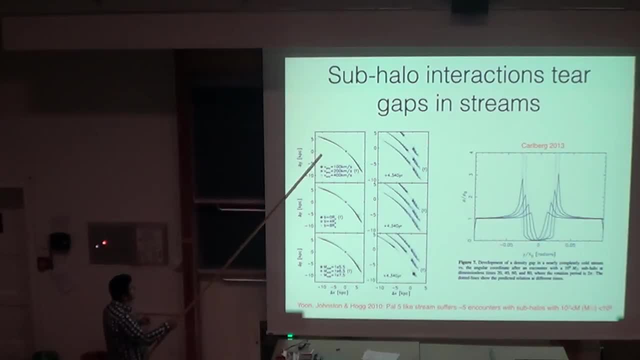 So here are simulations by Jung, Johnston and Holt. So this is unperturbed streams, And on the right panel These are streams perturbed by sub-halos flying nearby, And here different velocities of sub-halos are used. 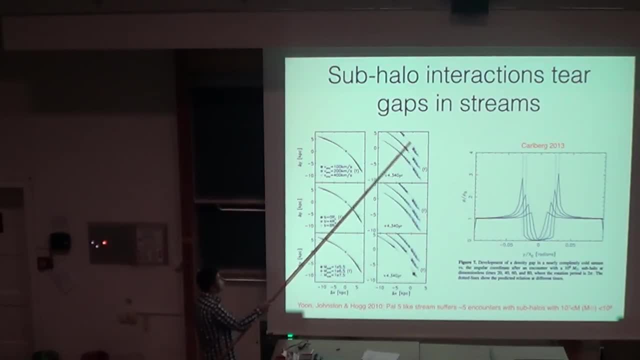 You can see that if you make the velocity really slow, the gap that opens is bigger. And here, for example, they dial up and down the mass of sub-halos. And if you make the mass quite massive, so a few times 10 to the 7, the gap opens really wide. 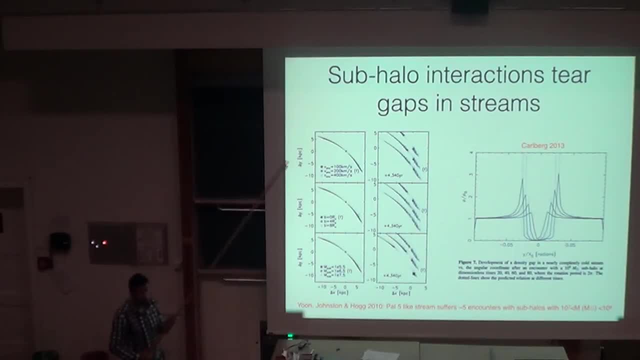 If you have a low mass sub-halo, the gap that's created is very narrow. In fact, there is a degeneracy between the velocity with which the sub-halo flies by and the mass, And that's because all that happens in this flyby is that the sub-halo imparts a velocity key to the stars in the stream. 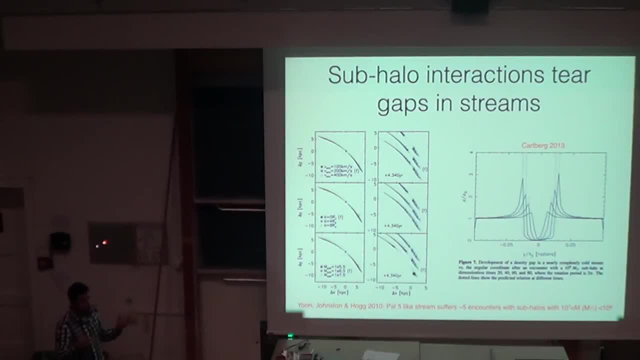 And so this is the integral of the acceleration. So if you have smaller acceleration provided by a smaller mass sub-halo, but you do it over a longer period of time, a longer counter, eventually you get the same velocity. So in this type of experiment there is a degeneracy between the mass and the velocity of sub-halo. 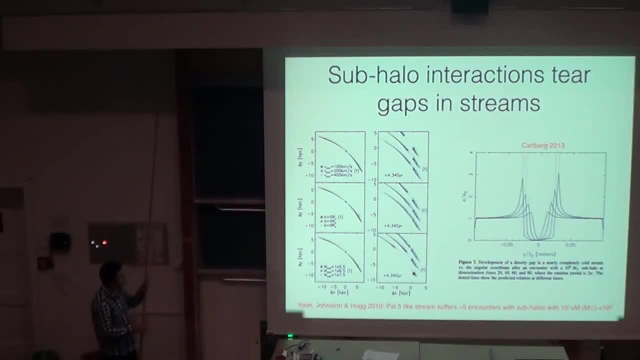 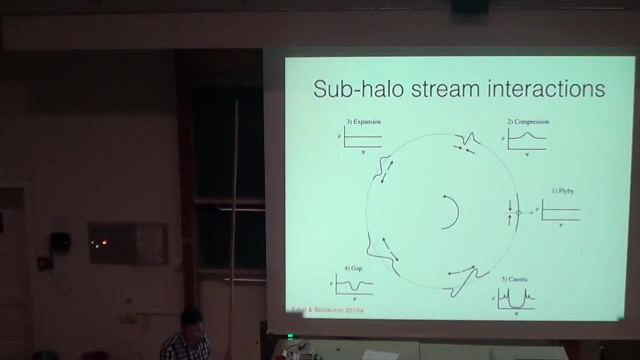 But an interesting, a very interesting pattern emerges. So these are profiles of these gaps, So these are star counts along the gap And you can see there is a hole in the stream, But on either side there is a density enhancement, And this is a paper from Carleberg et al in 2013.. 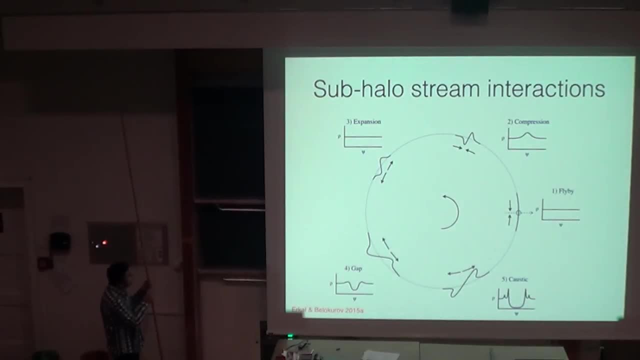 So Dennis Urkel developed a very comprehensive, very clear picture of what actually happens. So here are different periods in evolution of the stream as the sub-halo flies nearby. So this is a unperturbed stream And the sub-halo flies nearby. 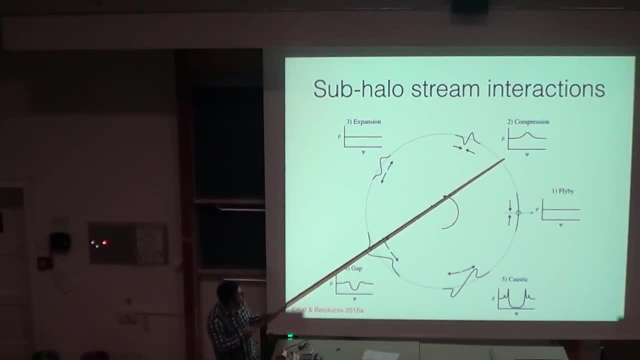 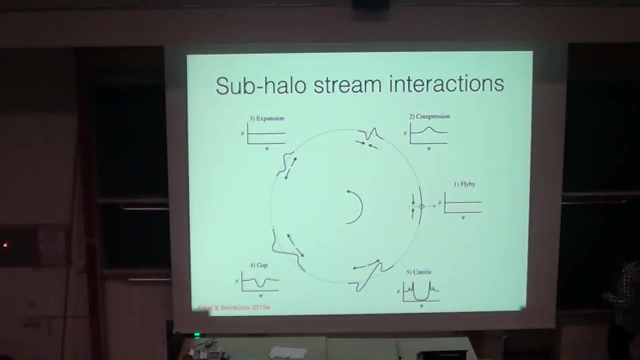 Nothing happens And then, very quickly, there's a small period when all the stars that felt the velocity go towards the center of gravity Right, And then they collect around the input point. So there is a small period of compression. But if you give a star a velocity that is higher than its current velocity, 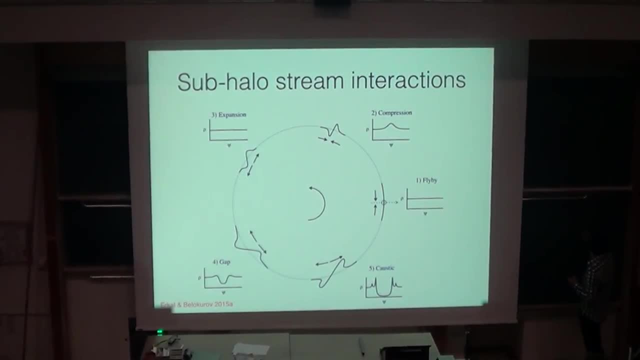 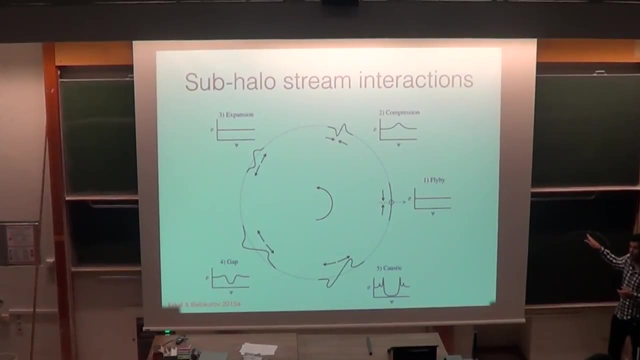 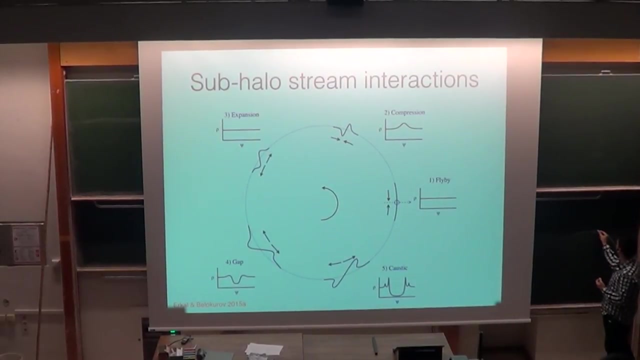 just what will happen? it will go on a higher orbit Right. So in the coordinate system that is rotating with the input point, this star will go on the. So, if you see the kick in this direction, it will go on a higher orbit. 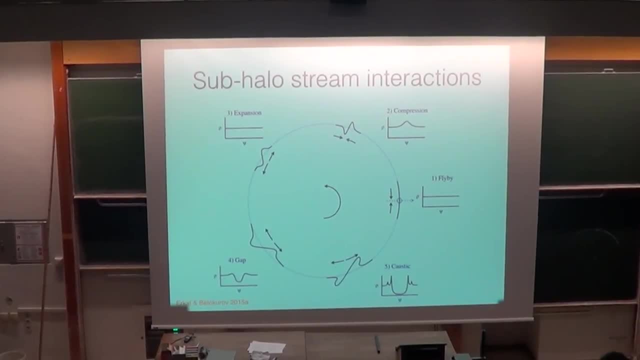 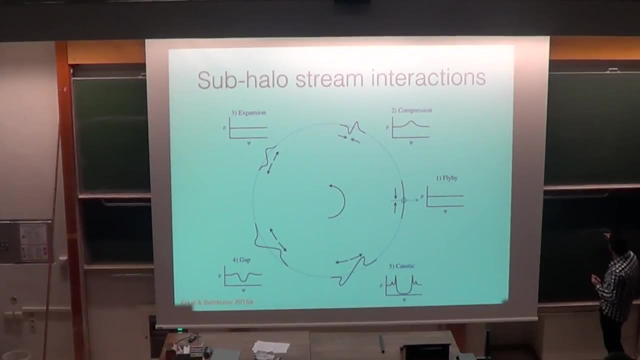 It will start to trail the input point Because on the higher orbit the periods are longer. as I mentioned before, A similar thing happened for the star that received the kick in this direction. So this is the input on the trajectory of the sub-halo. 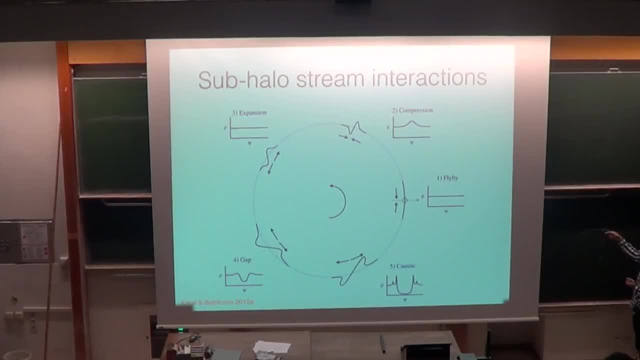 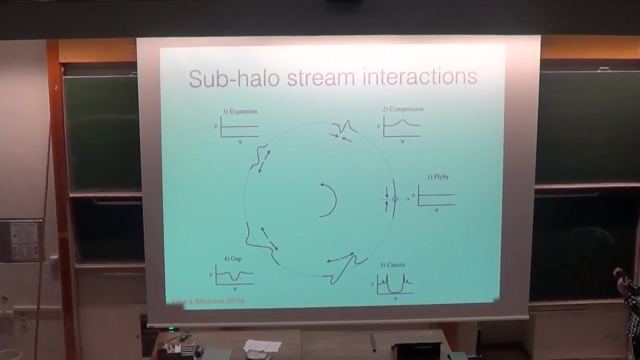 So for the star that is also moving in this direction but received the kick in the opposite direction, it will go on the lower orbit and will be leading the input point. So even though stars try to conjugate first, near the input point they quickly reverse. 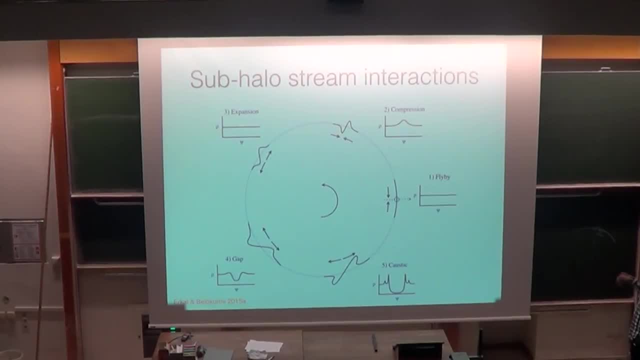 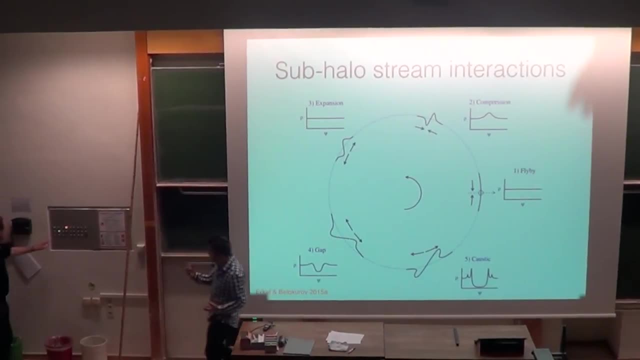 their motion and they go away from the input point, And that's why the gap opens. Of course, the amount of the velocity extravagantly increases, Right. So the velocity extravelocity, this velocity t-amplitude, depends on how far the star has. 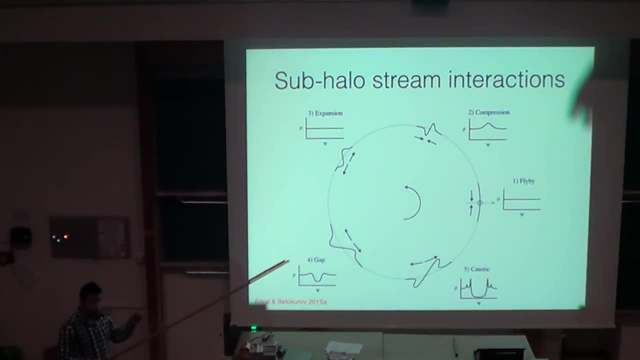 walked from the input point, And so some stars received higher velocity kick than the others, and they will start to overtake. So there will be a pile-up of stellar density on either side of the gap, And that's what is shown here. First the gap opens and then there are higher densities, these caustics on either side. 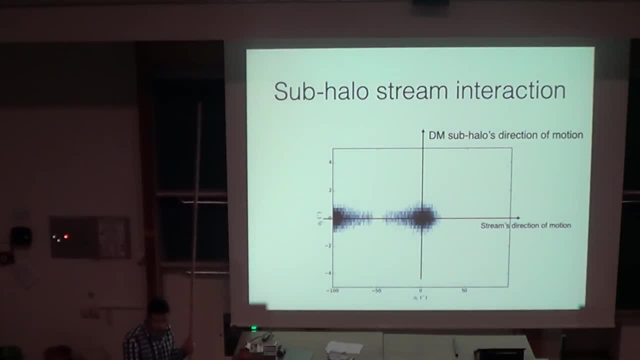 of the gap. I'll show you a quick animation of how this works. So here's the stellar stream. This is the stellar density, And it's actually a very long, very cold structure, but it's been spread out in a wide direction. 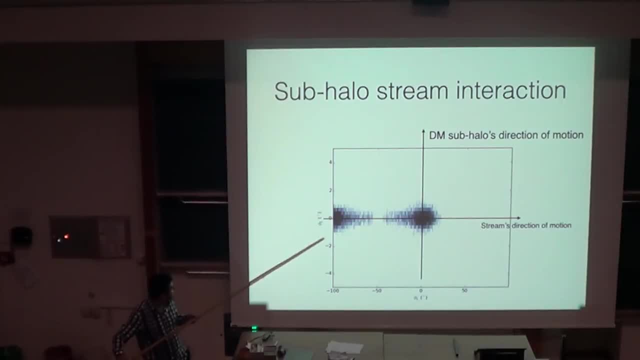 So this is just 2 degrees across the stream and 100 degrees if you pay attention to the axis layers in the longest stream direction. The stream moves that way and the sub-cable lies behind it- perpendicular. This is an in-decorative system that moves along with the stream. 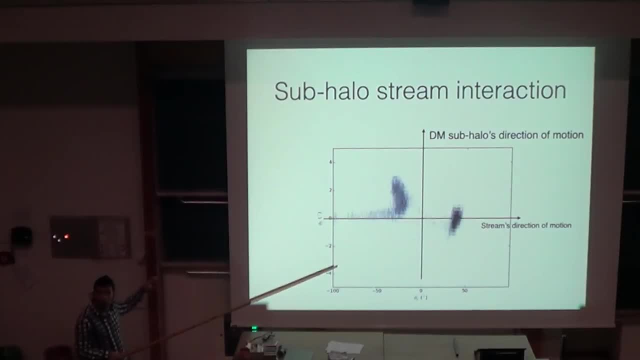 That's why you see this excited wobbling up and down And you can see how this region is evacuated and the stars start to pile up on either end. This signature is very unique and very particular And this imprint of the interaction is very particular in every phase: space coordinate. 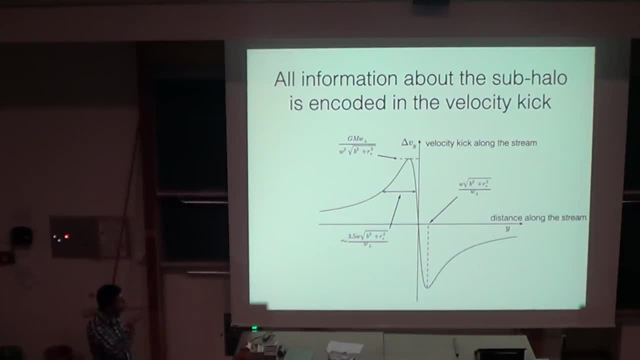 of the stream And it depends solely on the velocity. And here is the velocity as a function of distance from the impact point, where it should be zero by symmetry And it should be zero at infinity. So it goes for some maximum. 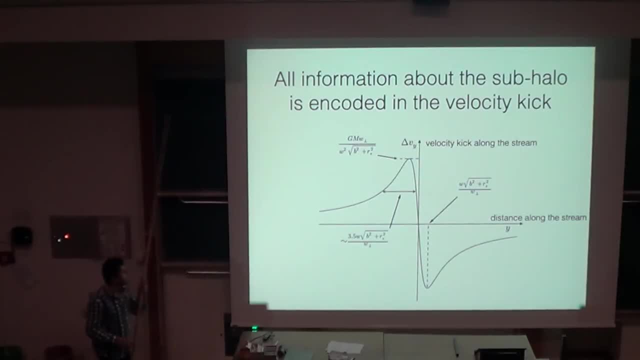 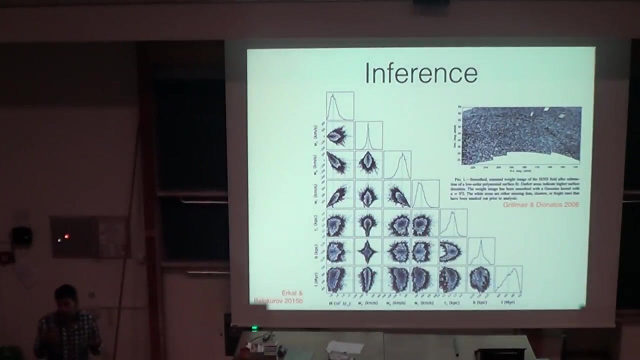 So there is a characteristic scale at which the velocity is maximum. So all the information about the sub-cable flyby is in this curve, in the curve that represents the velocity as a function of distance from the impact point. We have actually done an experiment in which we generated streams, created signatures. 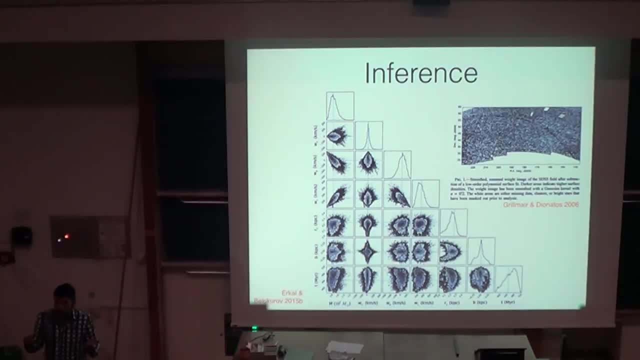 into sub-cable flybys and then with the smoke data, basically we observed the stream with Sloan LSST, DS Gaia and tried to measure the properties of the sub-cable And what we show is that if the perturbor is completely dark, it has the mass of 40. 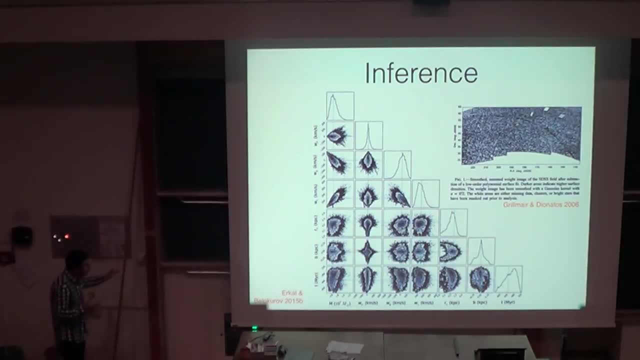 degrees And if the temperature of the sub-cable is slightly higher, you can infer all its properties, including mass and all three components of the velocity: the scale, radius and the impact parameter, and even the time of flyby. So I think the time is right now to go and follow up these streams that we know exist. 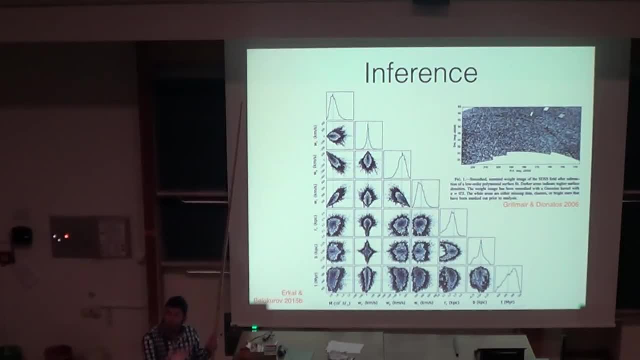 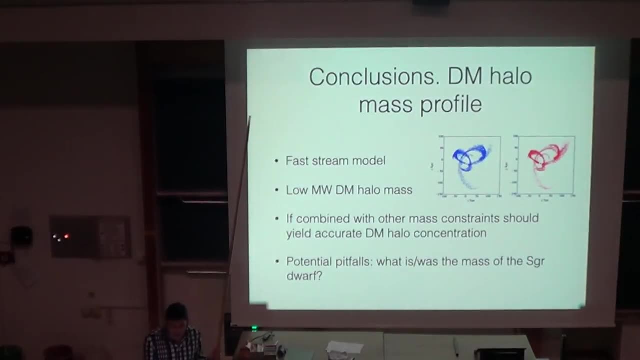 like the GD1 stream and try to find these signatures, because we now know how to infer properties of dark matter sub-cables. I have conclusions, but I think I more or less gave you the conclusions as I went along. So the important thing: we have fast stream models, we know how to generate streams. the 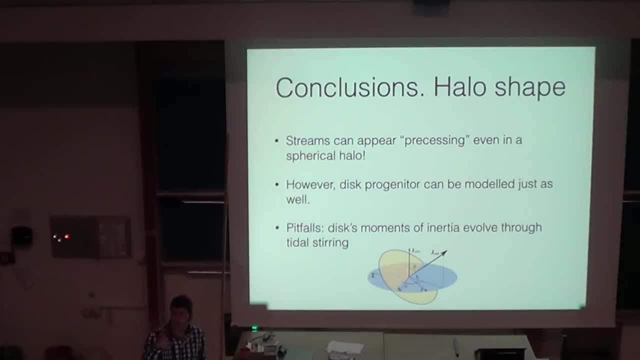 stream production can be extremely complicated if the dwarf progenitor was not a simple pressure supported system. But there is interesting information that is encoded in the precession of these streams too, So we can extract it, I hope, and learn about the shape of the dark matter- halo. 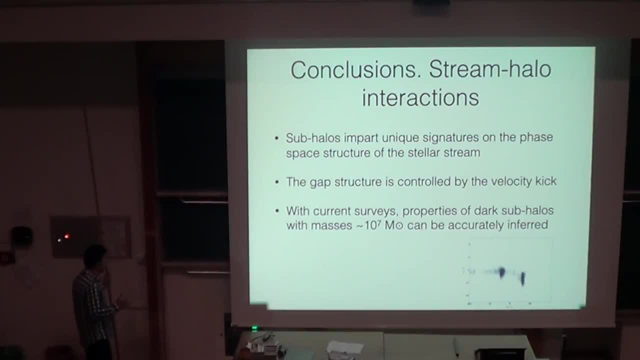 And probably the most exciting is we now have a clear insight into how the gaps form in streams, that gaps are not just holes and schemes. they have very particular signatures in all six projections of phase weights. So if we have an undeniable signature from the flyby, we know now how to measure the. 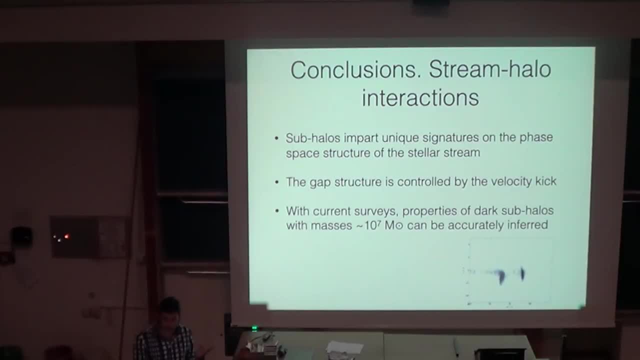 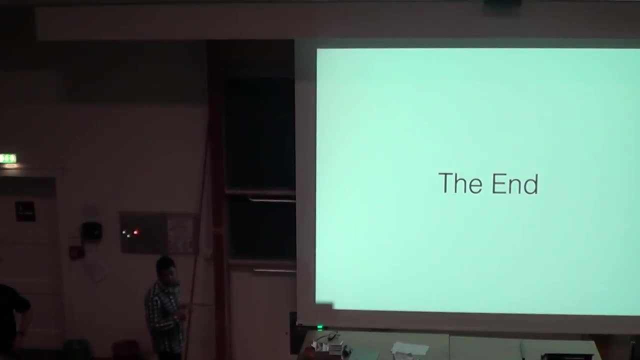 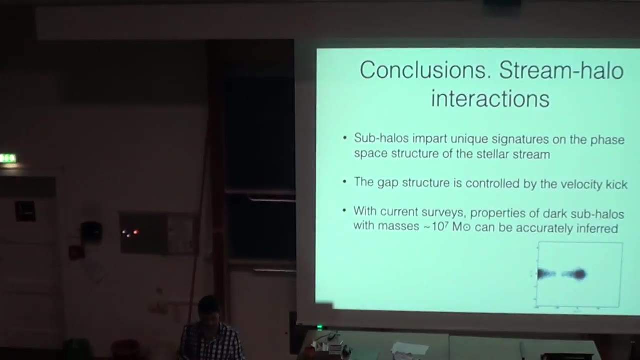 Yes, Yes, Yes, Yes, Yes, Yes, No, No, No, No question The last two questions you want? Yeah, Sure, So you showed up earlier on the slides in this: There's, there's humans野. whoever is nerd. 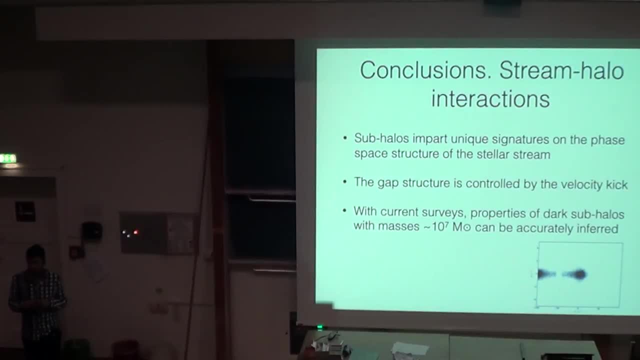 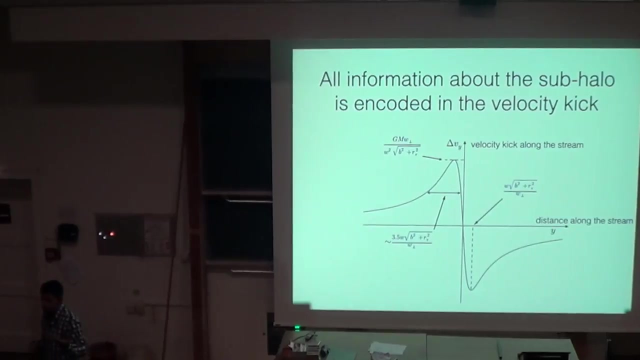 You're not an Deal A lot, Yeah, Yeah. What can you say about That's it? So how is Yes? What do you expect the reconstruction to look like? So, as I said, all the information is in the shape of the velocity kick as a function of distance along the stream. 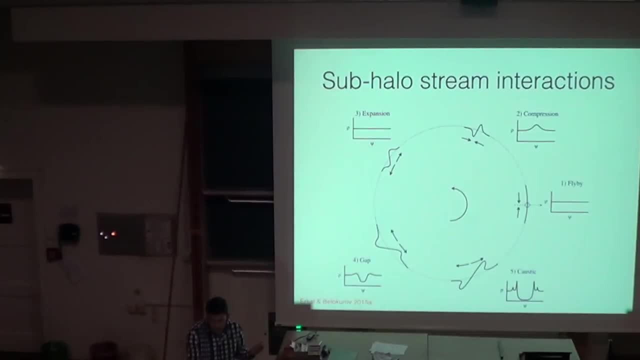 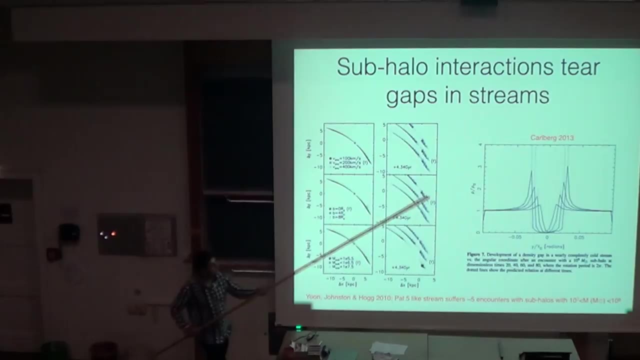 So this shape will be slightly different and, as a result, this shape will be slightly different. So this is: the density profile of the gap will be slightly different, So you will have to model it if you want to extract this information. But that's probably going to be quite difficult. 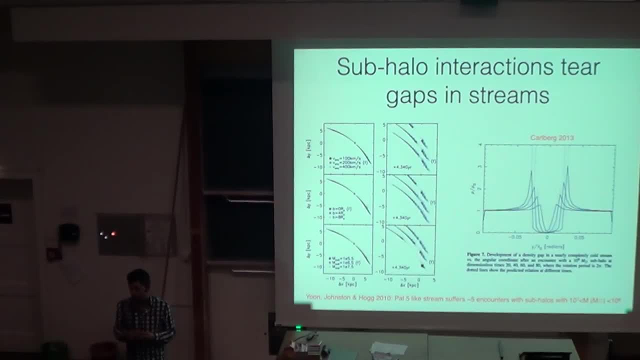 So a slightly symmetric assumption is probably fine for the moment. But yes, if you have very accurate measurements- and basically what you need is lots of stars to measure the density evolution quite well, you could probably tease out progress. So you can see the properties of subhalions like ACO, ACT, or whether they have cores or cusps and so on and so forth. 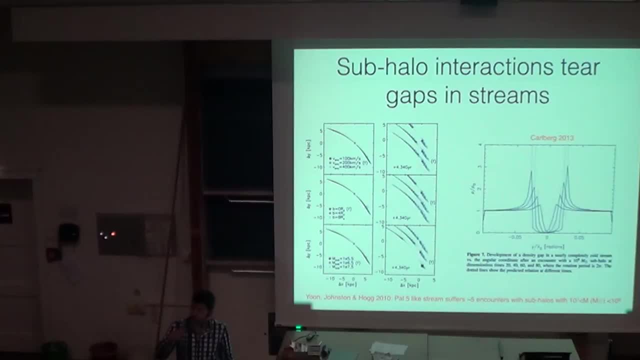 So it's all encoded in the structure that the flyby creates. It's like you use stars for tomography of the subhalion. Essentially, stars fill the pool from the subhalion. If it's extended then they will still fly to a different pool. 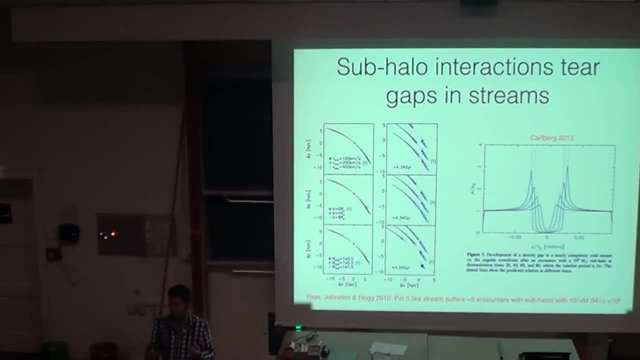 And if it's extended in an interesting way, they will start moving forward. They will move through the pool in a particular way, which will be encoded in the shape of the gap. So I think it's a dreamland, But, yes, you could maybe tease out this. 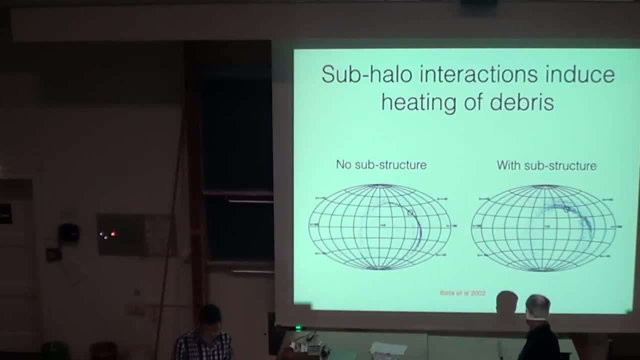 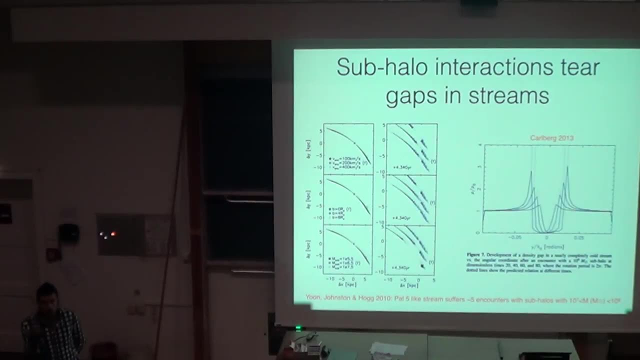 Yes, I haven't, But someone else did. I think it says there: June, Johnston and Hall calculated that there will be five encounters with typical PAL-5-like streams over its lifetime, with subhalions of over 10 to the 7.. 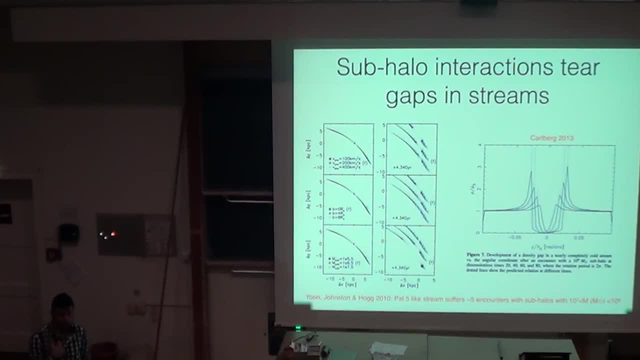 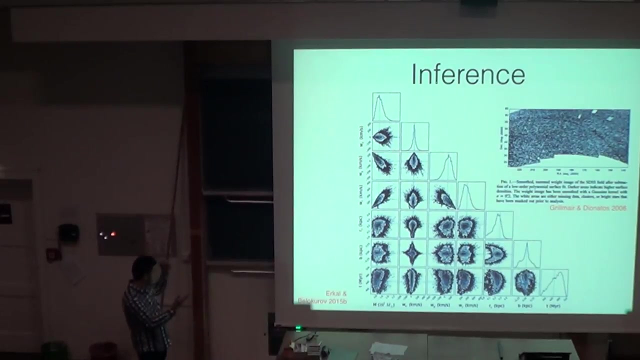 You mean the streams that we have. Yes, This is the stream. It already plays a role. I personally think that if you look at this picture, which is the best cold stream, the longest cold stream we have, you can already see lots of gaps here. 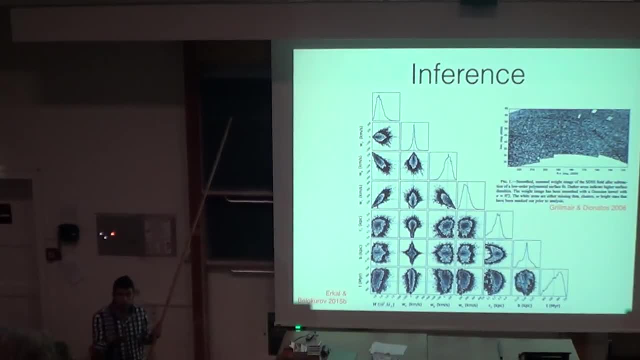 But I personally think that those gaps are to do with data quality issues rather than with sub-cable flybys. So what we're trying to do now is to go to telescopes with wide field cameras and say: let's follow this up and let's see whether these gaps are real. 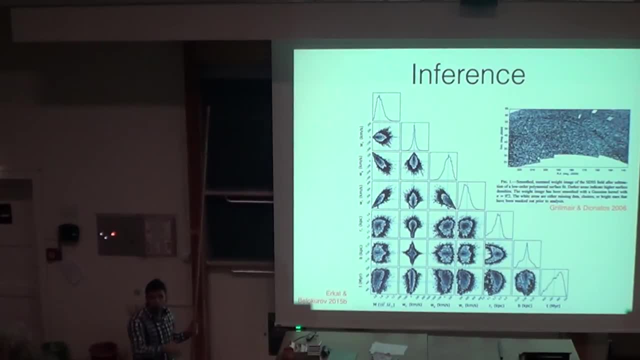 or are caused by bad seeing or clouds on the night when the alterations were taken- Something to do with star-tropical separation and sub-cable flybys. So I think we're now in a position to see if this exists or not, But I think it's slightly early. 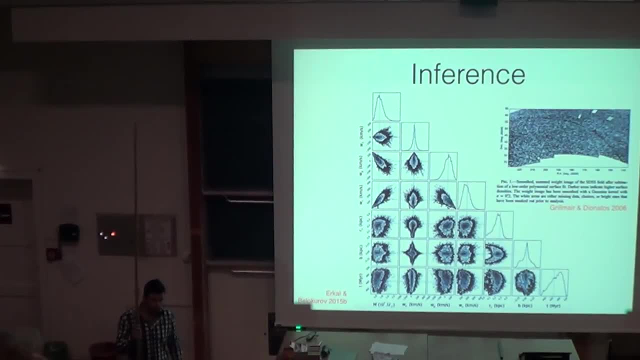 Ask me again next year. Further questions, questions. Okay, then let's open. I'm going to do an experiment. I'm going to get the microphone. Maybe that's actually useful. The question: askers can use better the microphone than me. 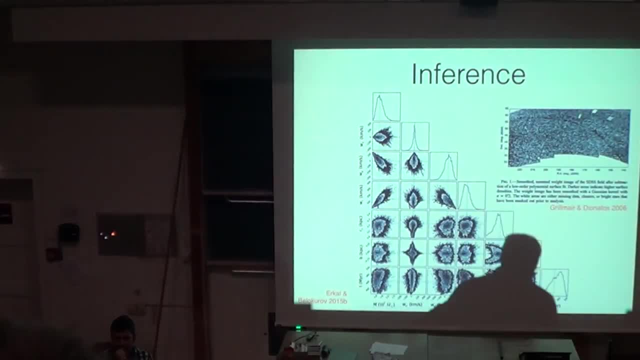 and I don't know what to do with it. Oh thanks, It's following the last question. So you said you had about five events for 105 during this lifetime. Yes, You are interested in the sub-cable mass function in the end. 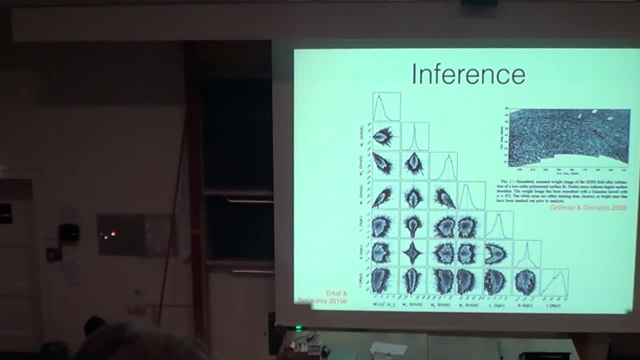 Yes, So what are the other candidates and how much events do you need in order to estimate with more or less accuracy the mass function between 10 to the 7 and 10 to the 9?? I don't know an answer to this question. 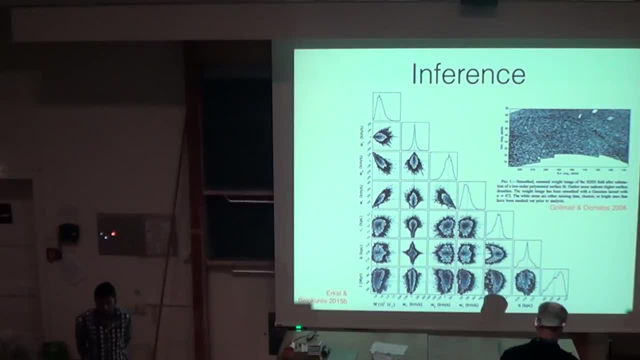 Because I think we haven't carried out this experiment. So we are at the stage where we want to find the signatures and try to confirm masses. I think this question is right. It's a good question: How many streams you need to follow up? 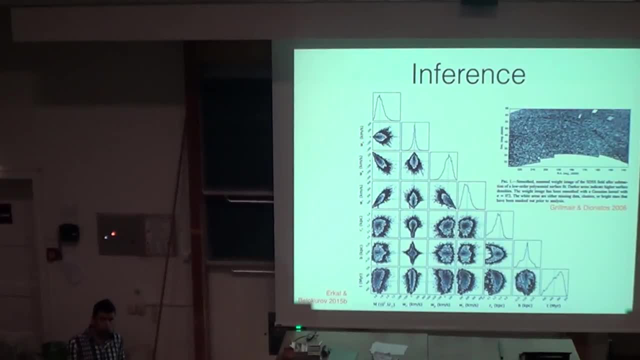 to constrain the mass function. However, before we do that, we actually want to move from this idealistic setup when we had a simple potential, a clean stream, which we peritoneally found sub-cable, fly-by, with the situation much closer to reality. 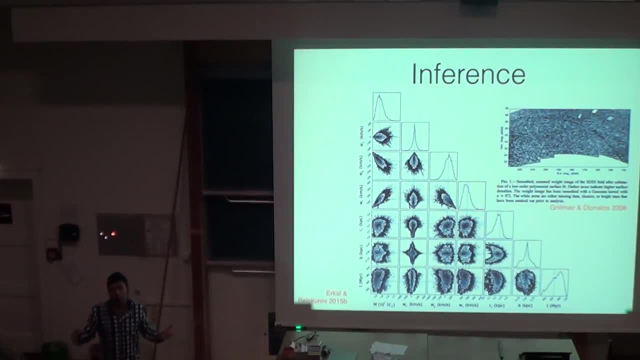 where we have a cosmological setup, the galaxy grows, sub-cables fly by, streams are peritoneal. What actually it will look like in that case will be probably much more complicated than that, So I think we want to address that question. 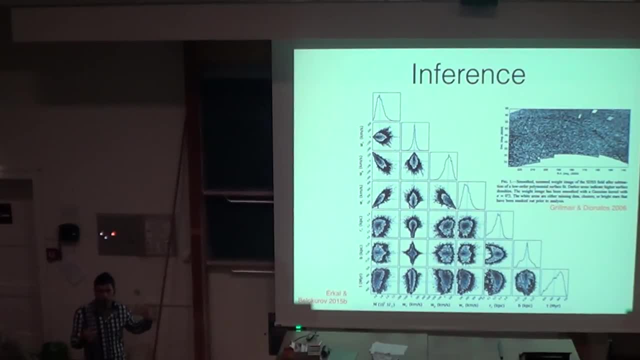 how to construct information from the illicitly peritoneal streams before we go and try to do the mass function, Because those streams probably have felt the dilution of the potential. So it's kind of, I think, too early, But I think it's a good question. 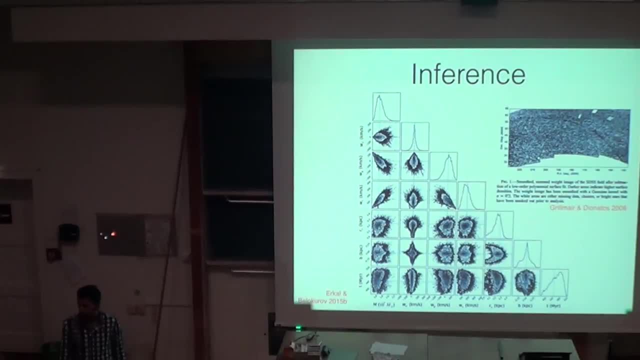 But I don't know yet the answer. The interesting thing here is that once you measure it, once you put constraints on the fly-by, not only you know the mass and the scale radius of the return, but you know roughly its trajectories of the velocity and the income current. 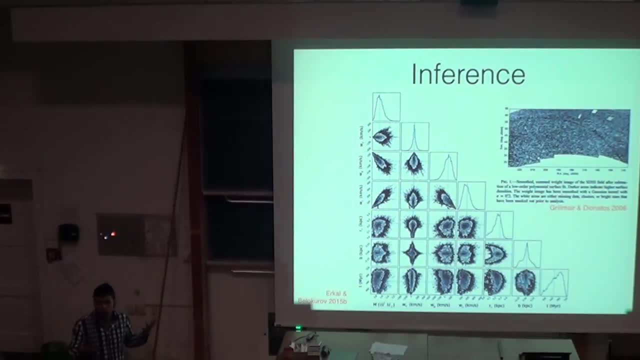 So you can probably start to rule out whether it was a dwarf galaxy that is known to orbit the Milky Way that would have caused it, Because the biggest signature would be from the most massive peritoneal sources. When you said initially that you can calculate the streams backwards, 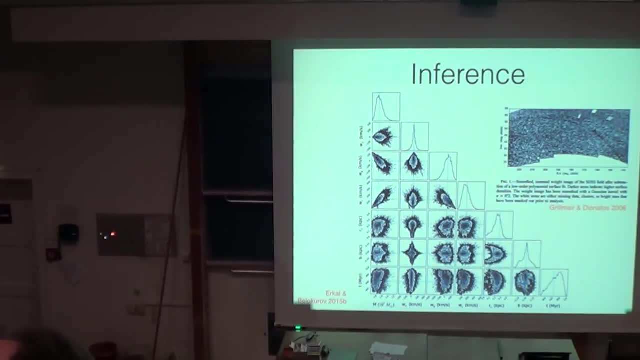 that makes the assumption that the potential of the Milky Way did not change dramatically in the past. several gigabits. Yes, How good is this assumption? I think this is a. I laughed when the speaker said this. It's a very interesting question. 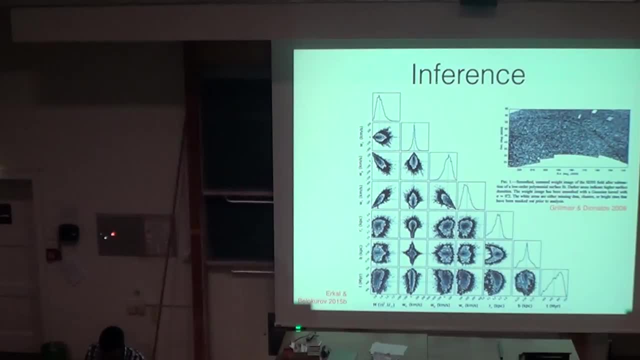 It's a very interesting question. It normally means that they don't know how to answer it. No, Or they're going to say something also, But I'm not going to do that. Well, I think it depends on the mass equation history. So in the Milky Way. I have very strong belief that the mass equation history has been questioned in the last few years. We have many lines of evidence that all agree that the Milky Way hasn't accreted much until the cloud fell in recently. 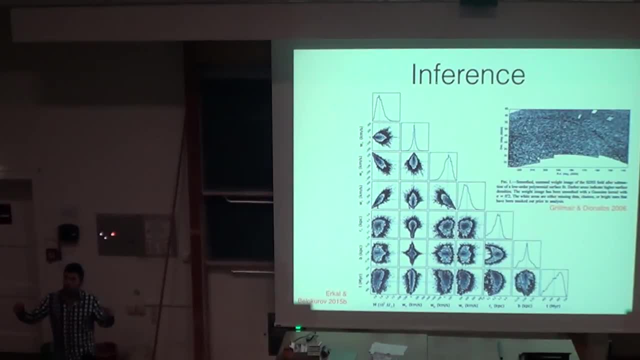 So there was a period of calm. In that respect, I think the last you know, six or maybe even eight giga years in the Milky Way were quiet. So this assumption in the Milky Way probably holds and I can explain why I can make this assumption. 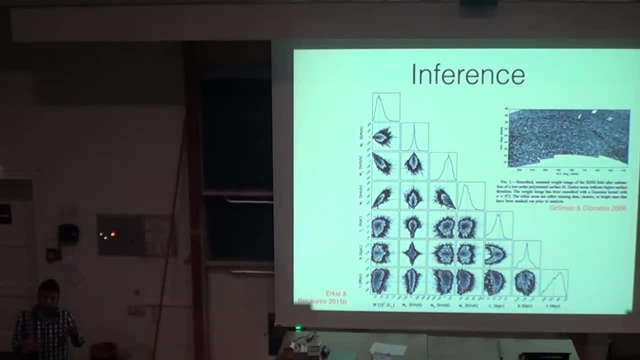 But in Andromeda that's not a good assumption And that's why we actually want to do this experiment of trying to model streams in cosmologically motivated setups. where this big potential holds, It need not necessarily be the accretion of new material. 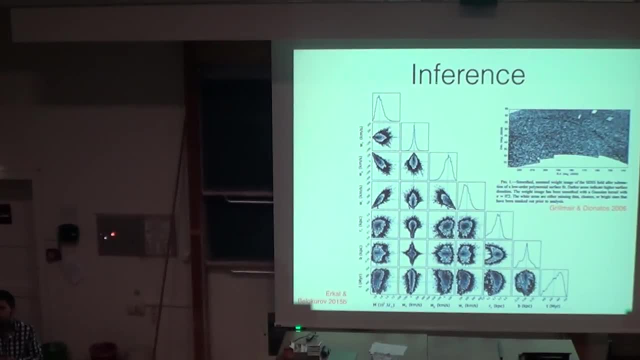 It could be tidal torques exerted by the Andromeda Galaxy, for instance, right. So the Andromeda Galaxy is probably too far away, and has been quite far away for a long time, to exert torques, But what I think has been shown to matter a lot, and it's only kind of came into the light recently is the Magellanic Cloud in the fall. So the Magellanic Clouds have always been assumed to have mass of more than 10 to the 10th of masses, which is interesting but not that scary. 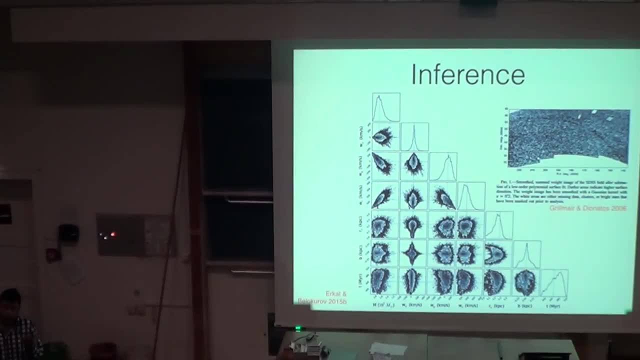 But recently there's many observational facts that point towards Magellanic Clouds being more LMC, in particular being quite more massive than that. so 10 to the 11th or so. So this is now slightly complicates the picture. 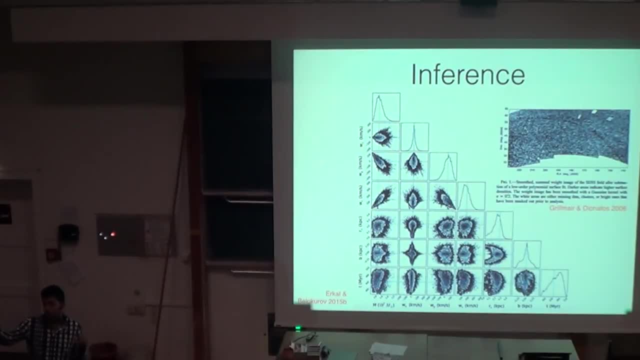 because the Milky Way will rebound as a reaction to the pull from the Magellanic Cloud itself. So everything will be perturbed. The experiments we have carried out to see how much effect this will, how much perturbation this will cause on the skin, 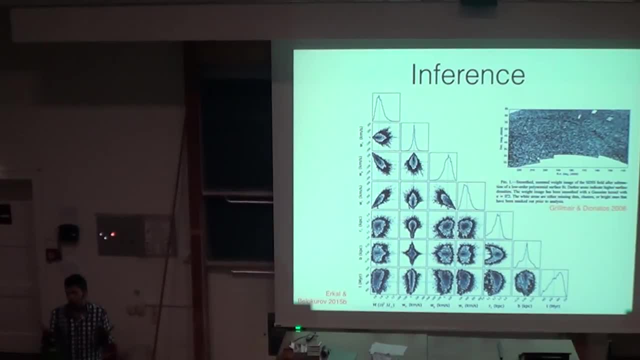 So far what we've seen is that it doesn't really change the picture dramatically. So the effect is quite small and we can think, But I think that's the only perturb that I can think of, you know, in the last few years. 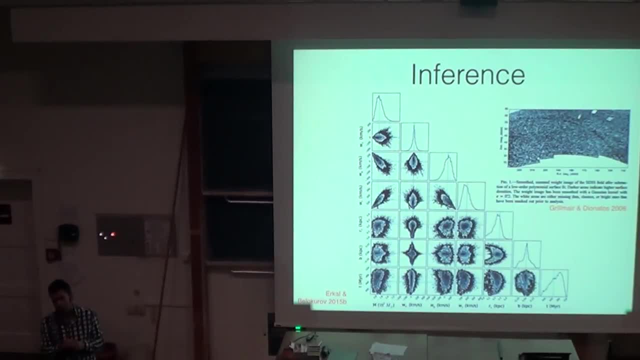 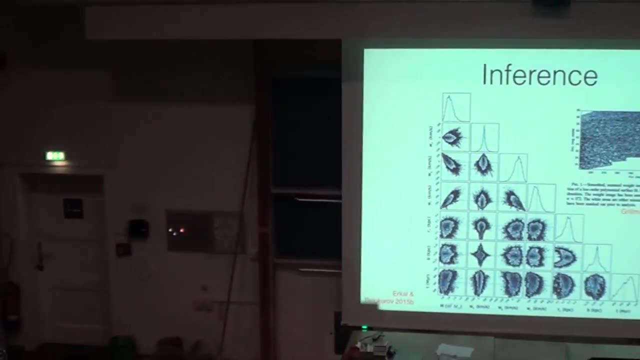 Otherwise, the Milky Way is actually a nice and quiet place. It's a boring place, if you want. So, coming back to the modeling, I mean you described this as a transformation between the different types of galaxies, but it will also. 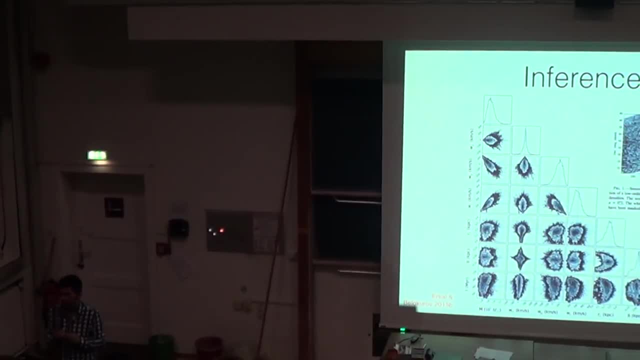 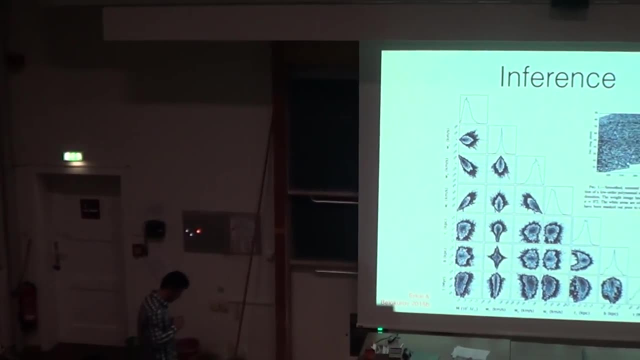 the modeling will also cause an increasing dispersion. So, for example, in branch A and branch B, or whatever you call them, the two branches- would this be detectable? I mean, I expect that the dispersion changes. Would this be a strong support confirmation? 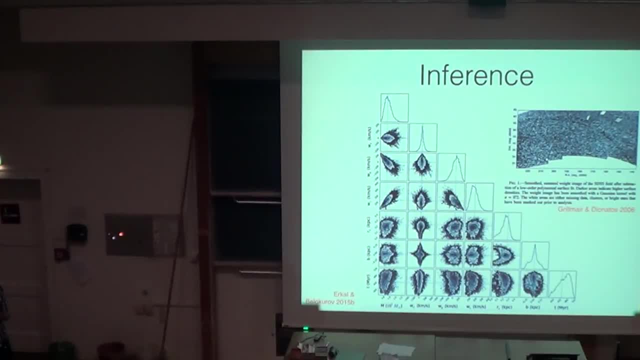 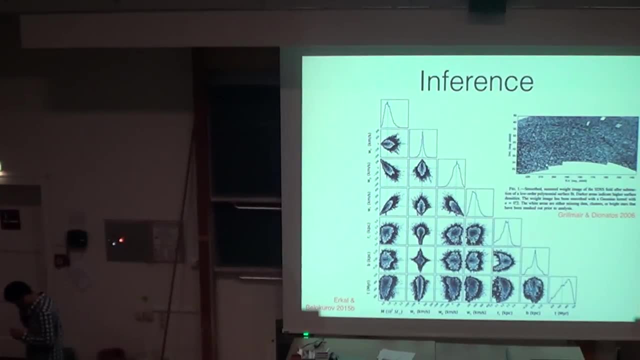 of this actually happening In addition to all the structural changes? Next question, But I think it all depends on: you're probably right, the dispersion will change, but the question is by how much? because the velocity dispersion of this thing changes along this thing. 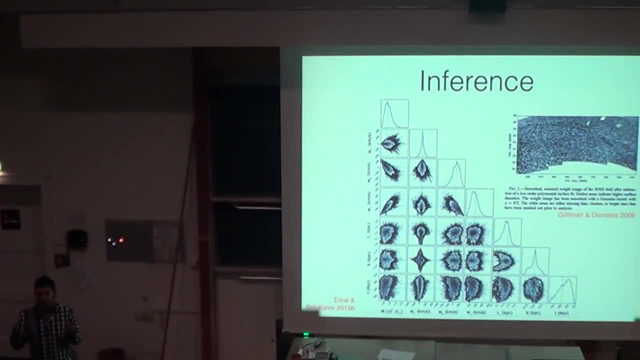 because there are these. basically, this thing stretches and compresses as you move forward, depending on the orbital phase of the degree. So there is no such thing as a velocity dispersion of this thing, right? So that already can be a change. 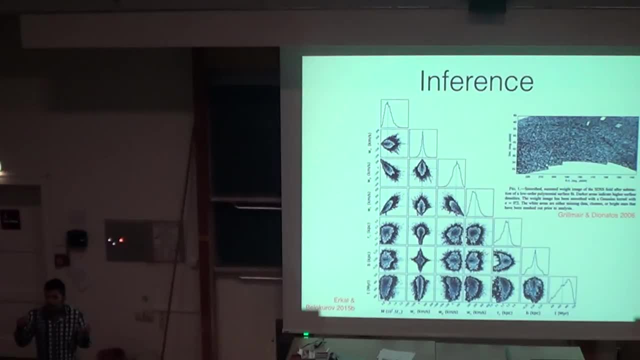 by a factor of two to four right. So I don't think the velocity dispersion changes due to essentially, you see, in the rotational component of the progenitor from different lines of sight, which is what is causing this different. I don't think this will be much bigger than that. 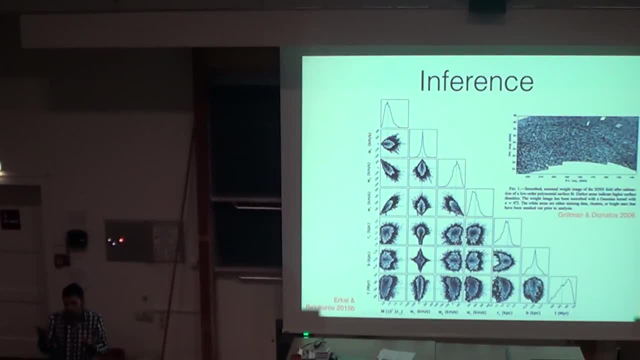 So it will be the same order of magnitude or less. So it will be very difficult to tease out, because you're looking at something that's constantly moving along this thing. So I think it's an interesting suggestion, but I think it needs to be tested. 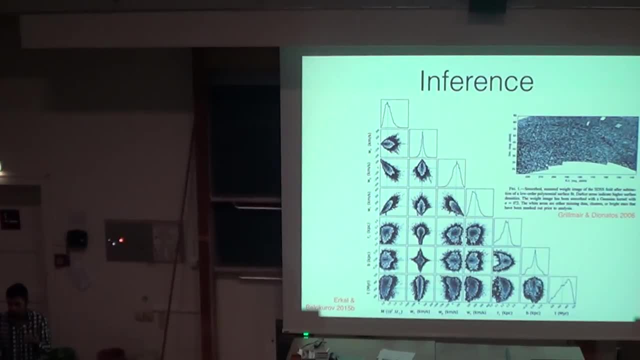 how this effect, what's the scale of this effect compared to the secular change of the velocity, dispersion of the degree? But I think it's an interesting point, So let me try to phrase this in a way that's answerable In part two of the talk. 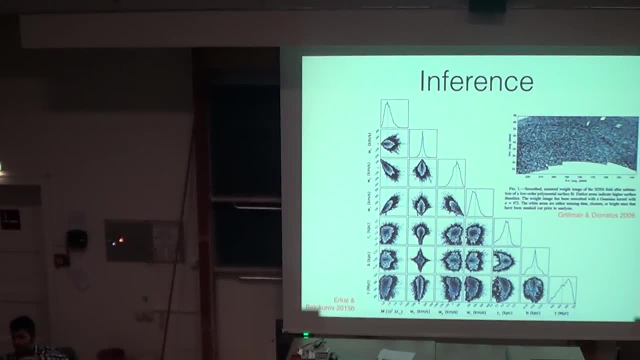 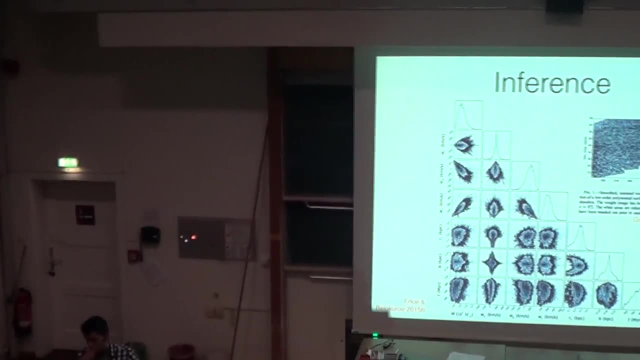 you said that the wobbles of the disc- It's possessive and wobbly- The random motion, the dynamical motions of the disc spread the stream out. In part three you say that you can put a lower limit on how. 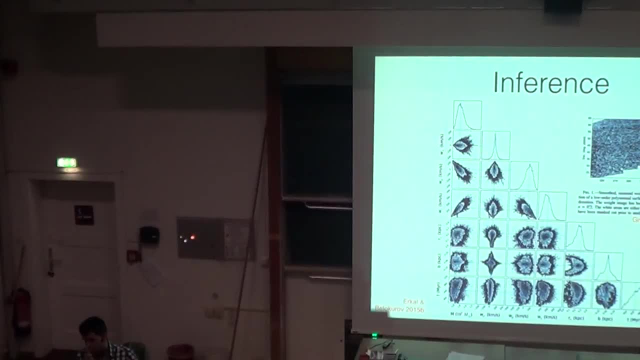 or an upper limit on how, a lower limit on how good a mass you can detect, But you didn't combine those two. The important thing is that these are two different streams. Sorry, I'll let you finish the question. Well, maybe you've just answered it. 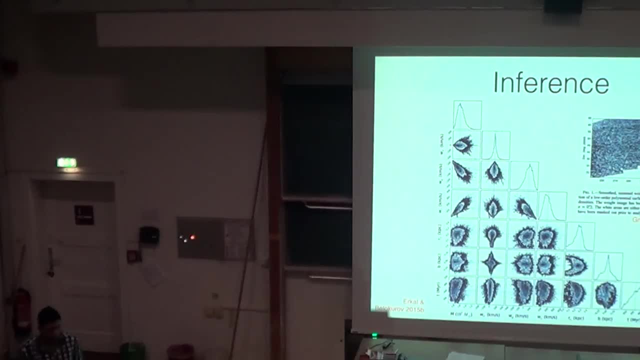 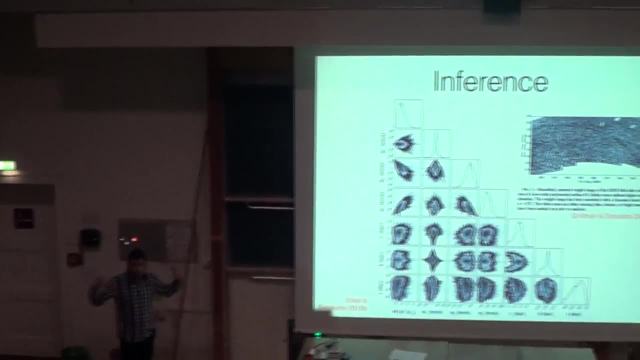 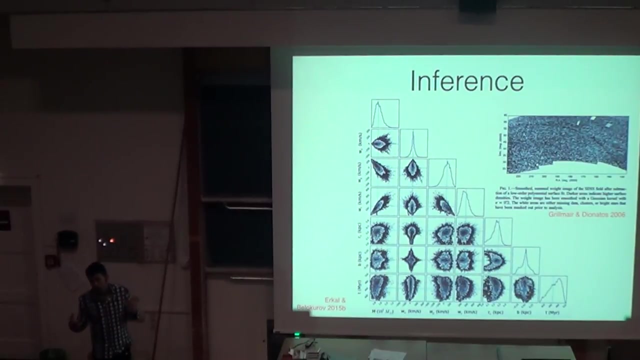 but isn't the wobbling going to make it harder to detect the low mass objects? So the potential, the mass and the shape of the angle overall, my suggestion is that we try to use the Sagittarius scheme for that because it's the longest. 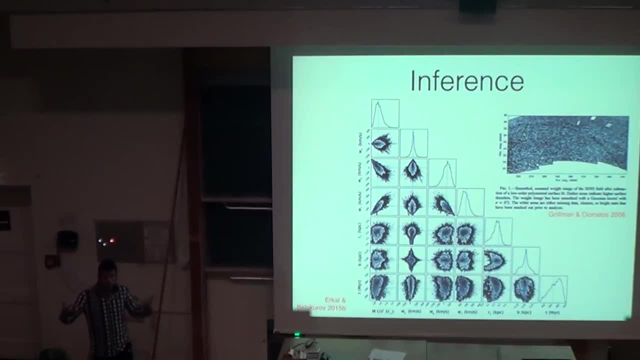 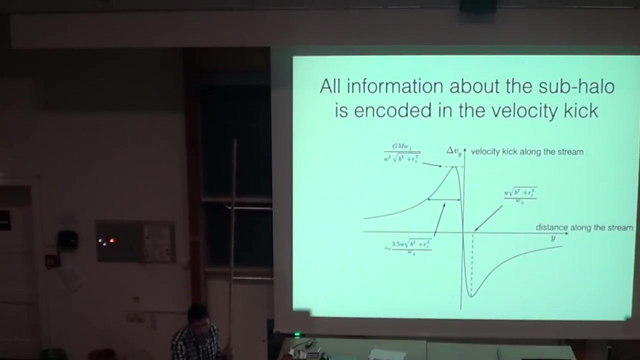 most luminous stream that reaches out to 100 kilometers per second. So it's the right thing to use The Sagittarius mass function. you need to see the difference. So these velocity peaks are really small, right, So you need as cold a stream as possible. 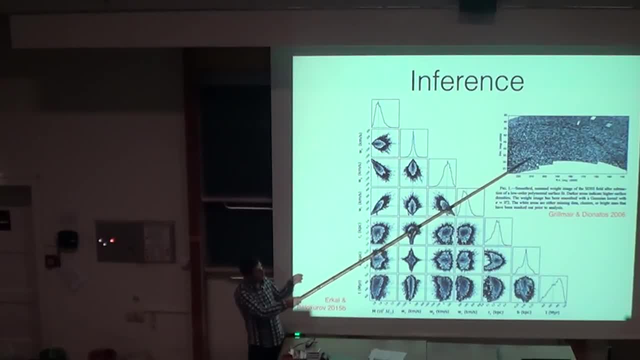 So I suggest we use globular cluster streams like this one here to do one thing and a big work galaxy to do the other, And so globular clusters probably do not abate as much. So I think the dysphoria in particular.